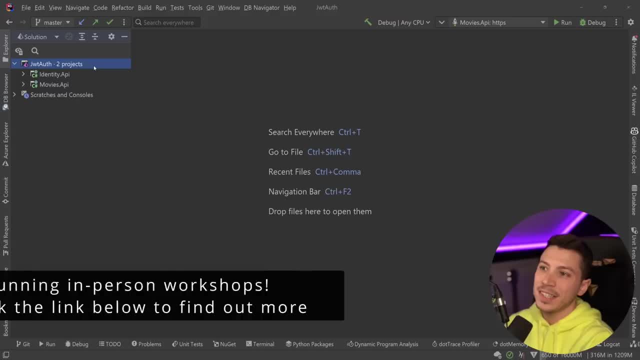 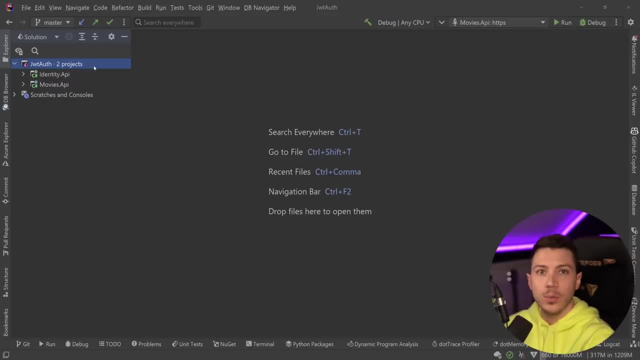 also tons of other videos going really in depth with the topic. It is a generic topic, it's not specific to ASPNET Core, and I want to focus on the implementation itself and show you how you can use it in a very nice way. Let me show you what I have here. I have this movies API and that's what. 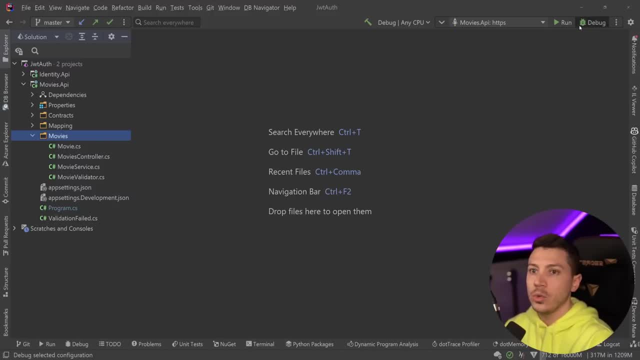 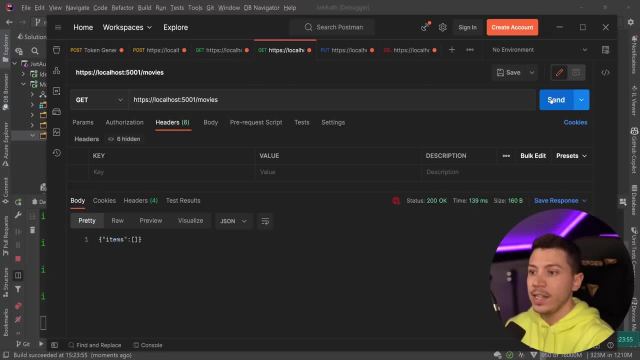 we're going to be dealing with directly in this video and I'm going to run it to show you what this API can do. So API is running. I'm going to go to Postman and we can list all the movies in the system. Now, unfortunately, we don't really have any, so what I'm going to do is I'm going to create 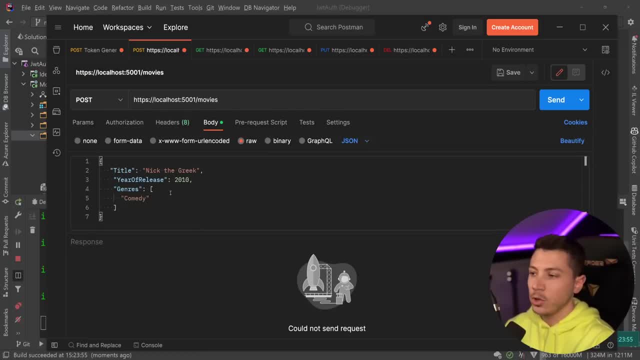 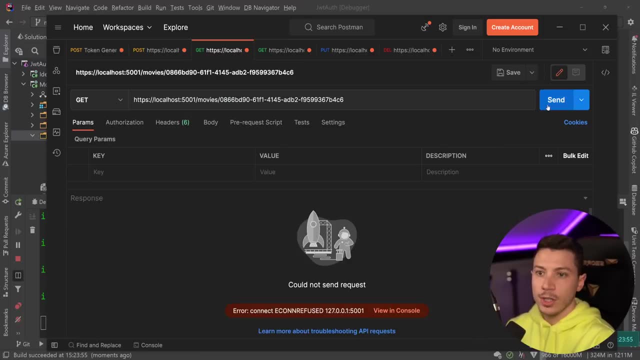 a new movie I'm going to create the famous comedy Nick the Greek all the way back in 2010.. So that is now created in the system. I can list it in that previous endpoint, as you can see, or I can get it using an ID Now. oh, I made a bit of a mistake. it's actually released in 2023 and it's also an 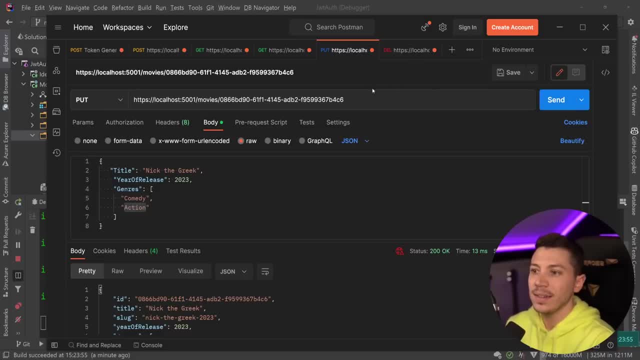 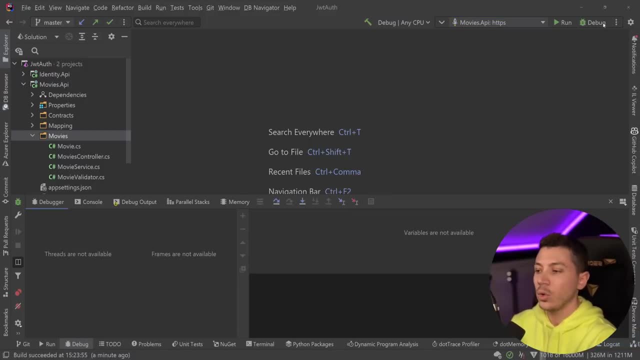 action movie, not just a comedy, So I can update it and in the end, I can simply just delete it. Now this API does not have any form of authentication authorization. I don't need to be someone or validate that I am someone to be able to call it. So my controller looks just. 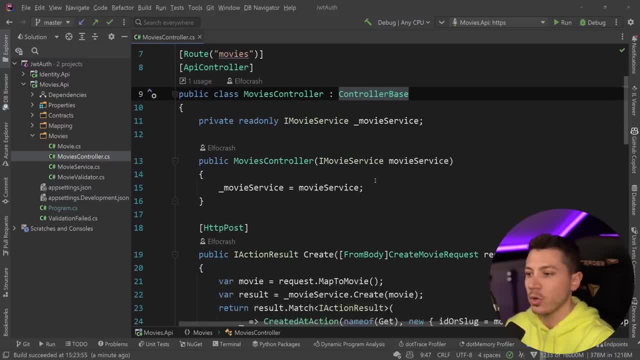 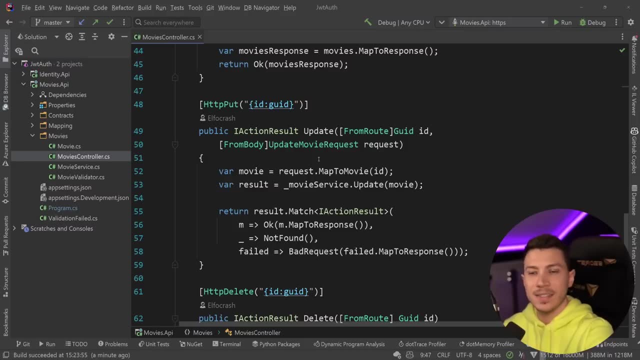 like this: I have an API controller attribute, a route implemented, the controller base, and that's how my endpoints look. Now, don't worry if I'm using controllers. I'm also going to cover minimal APIs in a second later in the video. So how do I add JSON Web Token support? Well, it all. 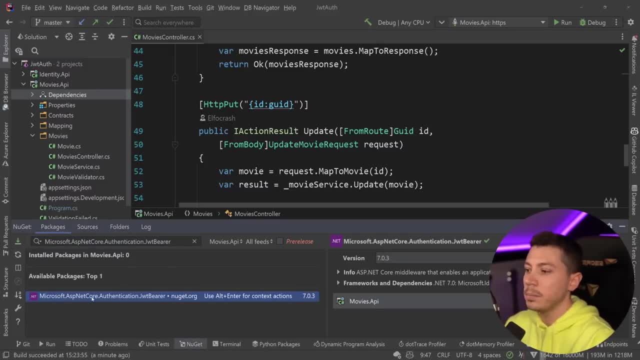 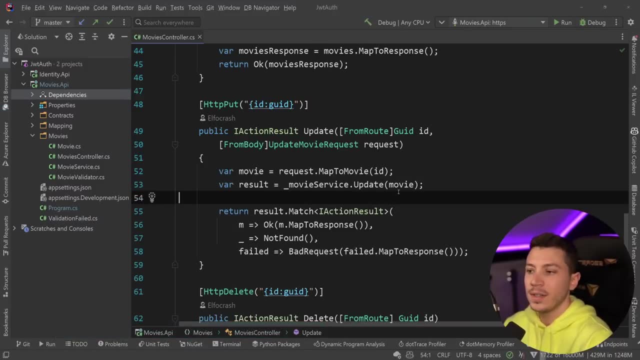 starts with a new git package. I'm going to go to new git packages and I'm going to add the microsoftaspenetcoreauthenticationjotbearer- And yes, I know it's pronounced jot, for some reason it's a w, but whatever, And configuration, thankfully, is actually pretty simple. It could be way, way. worse. So the first thing you need to do is to add a new git package. So I'm going to add a new git package And I'm going to add a new git package, And I'm going to add a new git package And I'm going to. 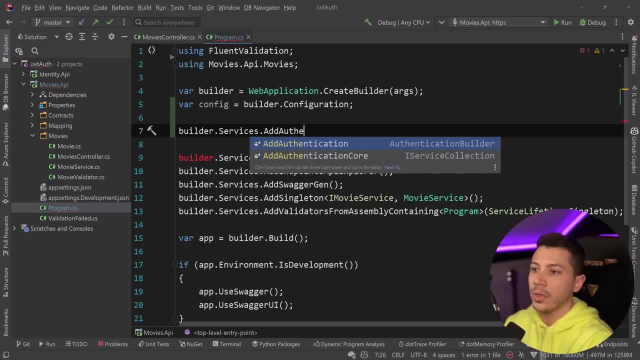 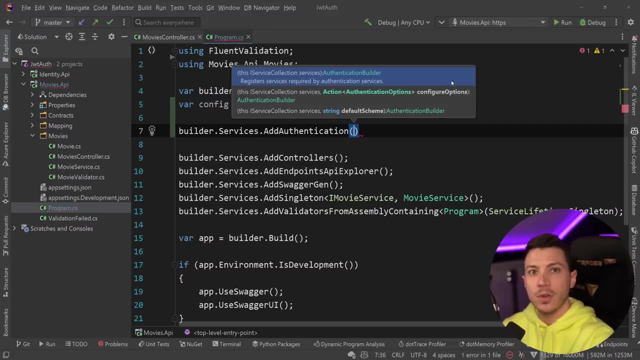 add a new git package. So the first thing you need to do is actually say servicesadd authentication. Authentication comes before authorization And just to quickly recap for the avoidance of any doubt: authentication is the process of verifying that someone is who they say they are, while authorization is the process of verifying that someone has access to what they say. 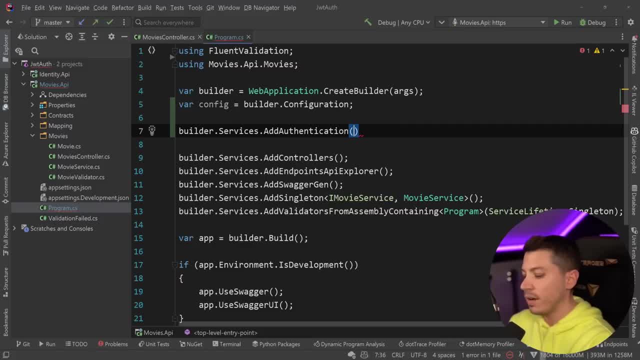 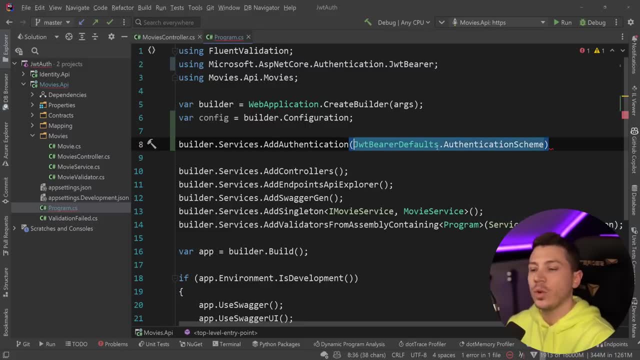 they have access to or just saying what they have access to. So now that we have this new git package, I can use the jot bearer default and I can use the default authentication scheme here. But another approach: if you want to just update your git package, you can do that by just adding a new git. package. But another approach: if you want to just add a new git package, You can do that by just adding a new git package. You can do that by just adding a new git package. And another approach: if you want to just add a new git package, You can do that by just adding a new git package. And another approach. 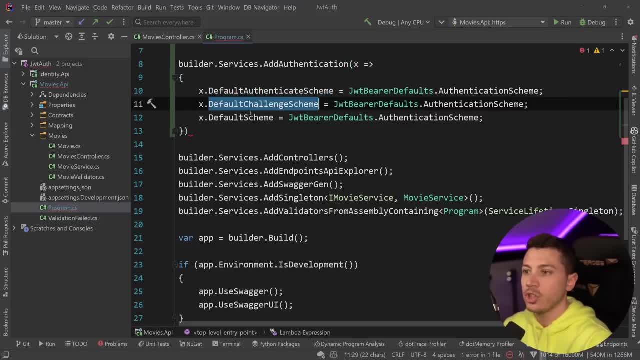 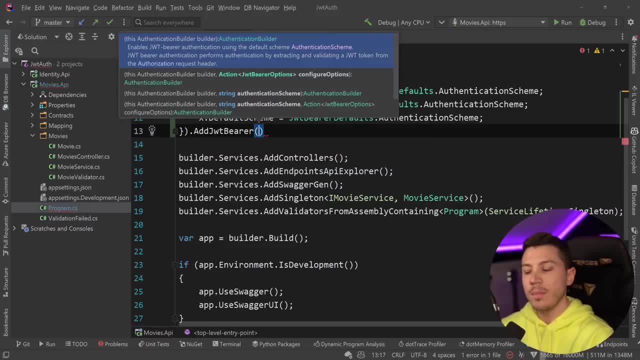 is to do something like this: You can set the default authentication scheme, the default challenge scheme and the default scheme all at once. And now, with that new git package, we also get this add jot bearer method, which adds the support we need. So in here we're going to. 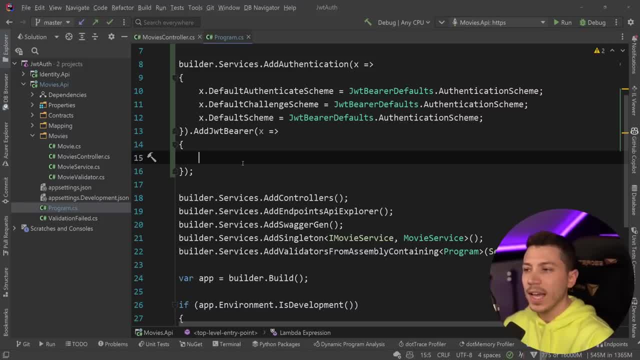 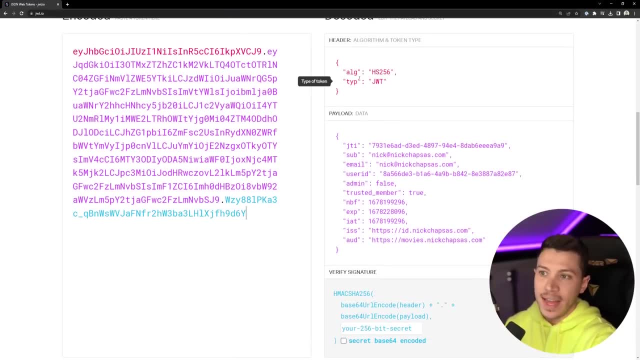 configure what we want to validate for our jot. And just to quickly recap what the jot looks like, here I have a jot generated from one of my own service- We're going to be taking a look at that in a second- And first we have the header, which contains the type of the token and also the 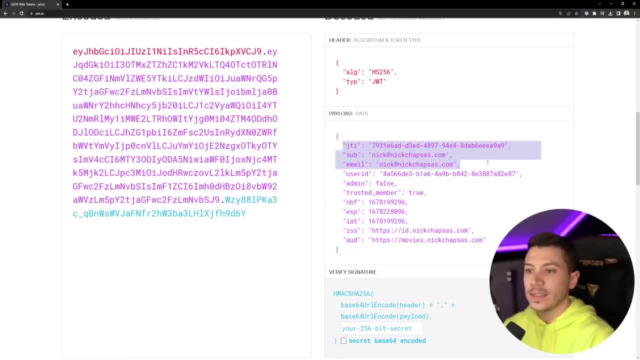 algorithm used to generate the signature. then we have a bunch of standard claims and custom ones. so json web token id is a standard one, same with subject and all of these ones over here. and then we have a few custom ones: email, user id, admin and trusted member, which i created, and then you have. 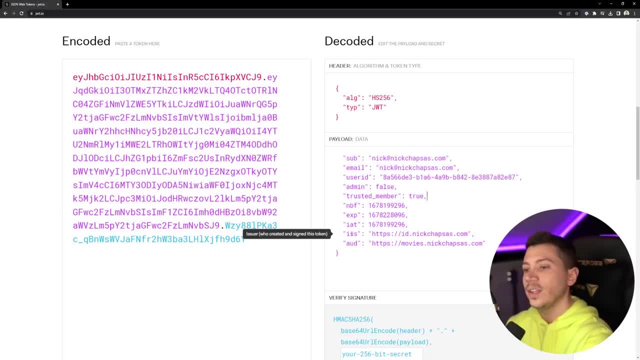 an issuer and an audience. the issuer is who created the token, and audience is who is this token intended for. so think of- i don't know, google authentication, creating a token for you to use in google slides. maybe you don't have access to google docs with that thing, so that token can only 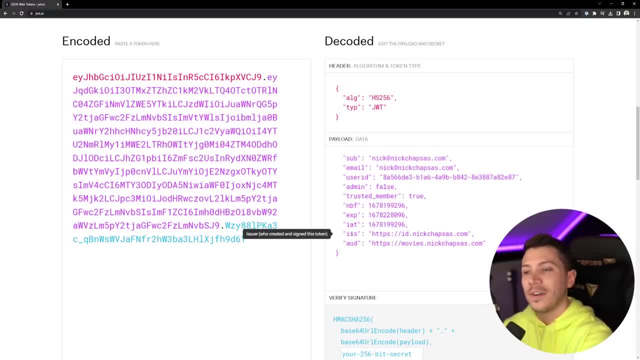 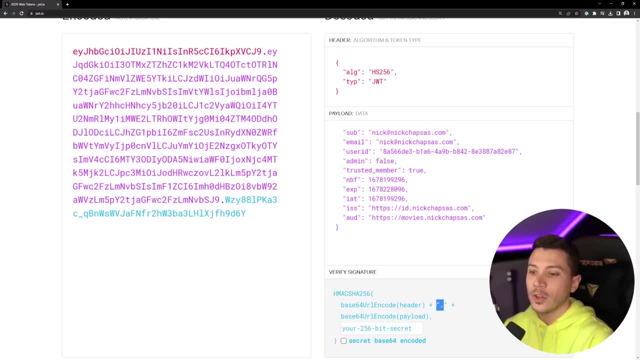 be used in google slides, even though it was generated by google and it is a valid token. and then in the end both the header and the payload are actually base 64 euro, encoded, separated with a dot. and then there has to generate the signature. hashing is not the only. 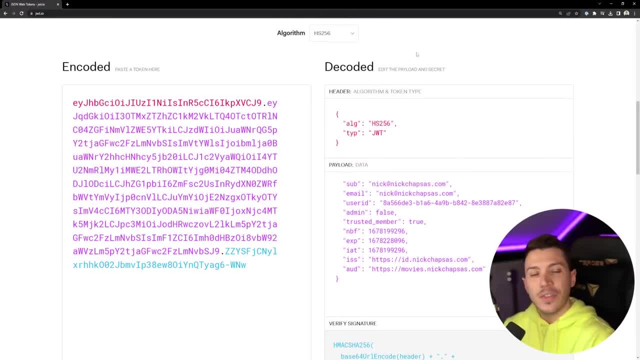 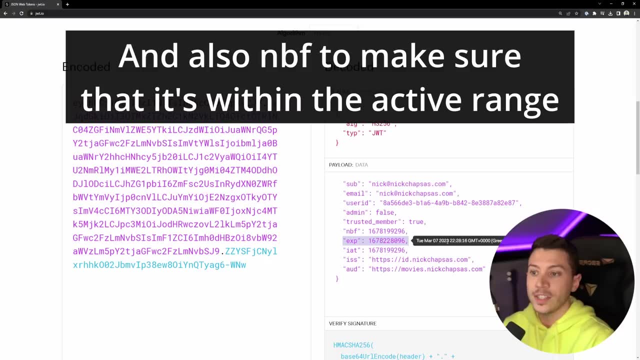 mechanism. by the way, to do this you can have public key cryptography as well, and other approaches, but this is by far the most common. so a few things you want to validate is the issuer, the audience and audience also that the token is not expired. on top of that, we want to validate the signature, that it is a. 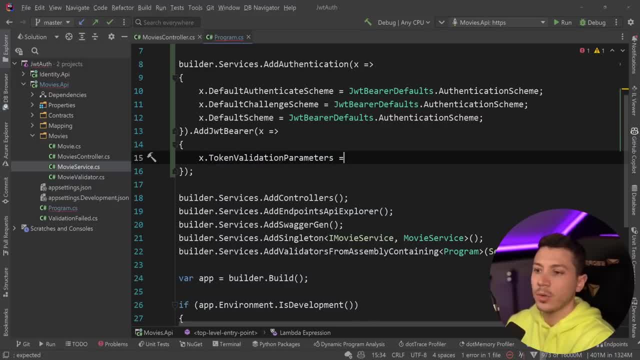 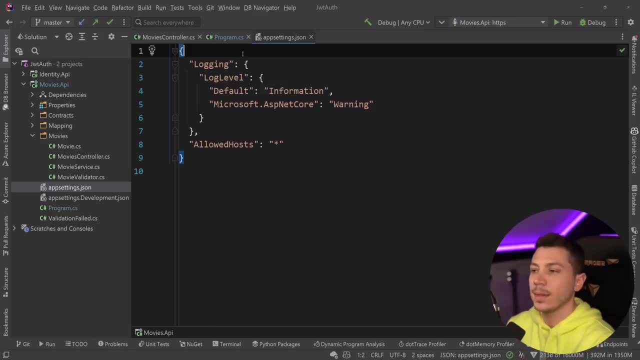 valid one. we can validate all that by configuring the token validation parameters value. we can create a new type over here, and what i'm going to do before i paste what goes here, is actually add some settings. so for the purposes of this video, i'm going to keep these here, however you would. 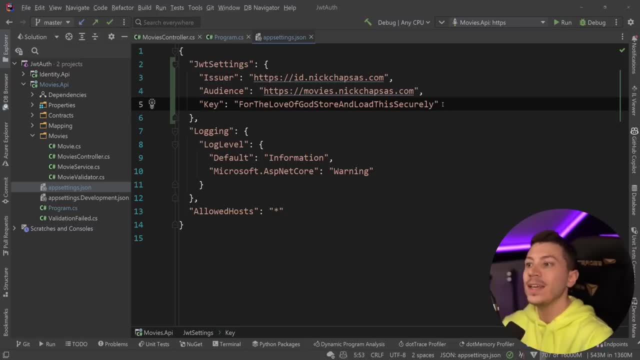 not store the key here. you would store it securely in a service specific design to store tokens like azure key vault or aws secrets manager if you want to know how you can store tokens like azure key vault or aws secrets manager if you want to know how you. 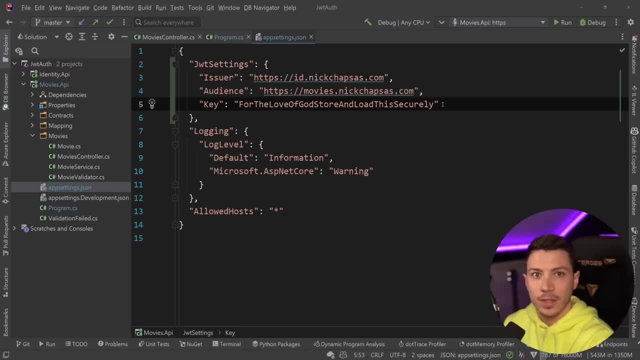 can do this with aws secrets manager- i actually have a video on that topic- but you should never have it in the settings like this. not only is it not secure, but if you want to rotate that token as the application is running, this limits you significantly. you have to redeploy and then you. 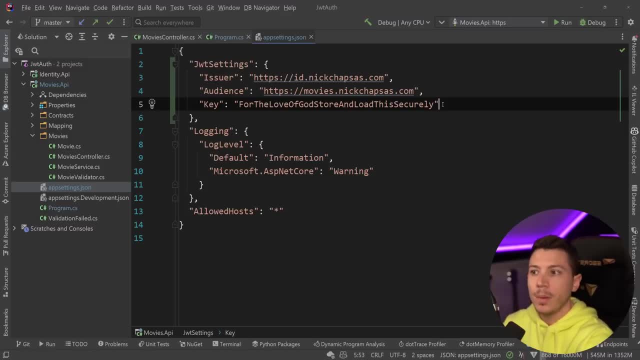 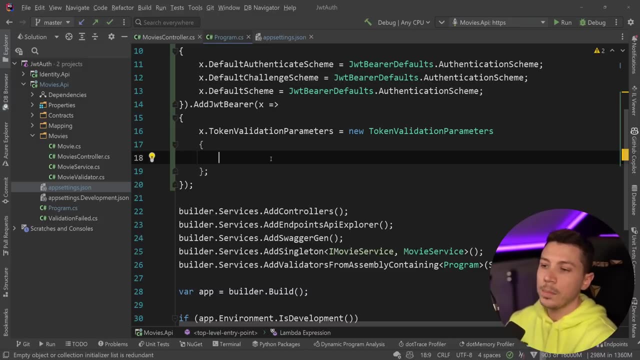 have to keep track of multiple keys, it becomes very tricky. but for this video i'm just going to leave it here, just so you can grab the code from the description and use it for your own purposes. so now, with these things set, i'm going to just show you all the parameters we have to specify. 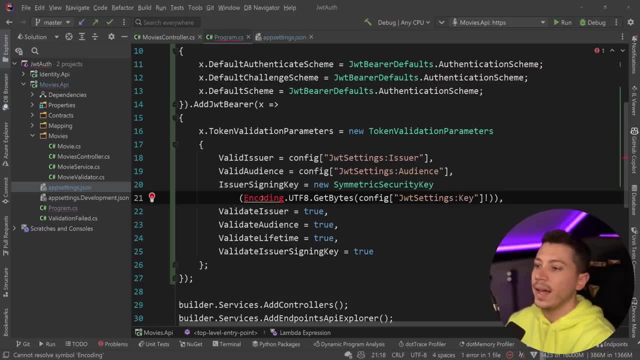 here, and these are sort of the minimum ones you need. so for this video, i'm going to leave it here, here, and these are sort of the minimum ones you need. so for this video, i'm going to leave it here. so we have the valid issuer, which we passed down from configuration valid audience as well then. 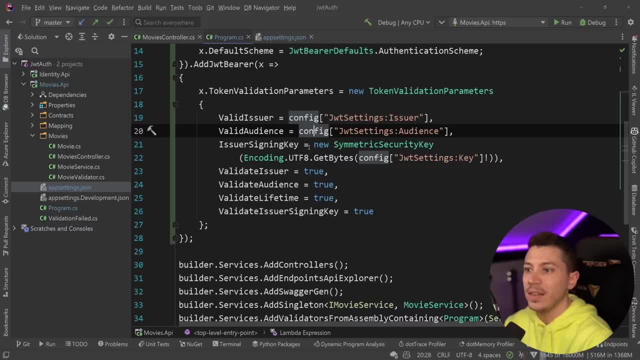 the issuer signing key, and that is a new symmetric key in this case, which we get from the settings. again, like i said, you really want to load this from somewhere that is designed to store and load these things. and then we say that we want to validate the issuer, the audience, the lifetime of 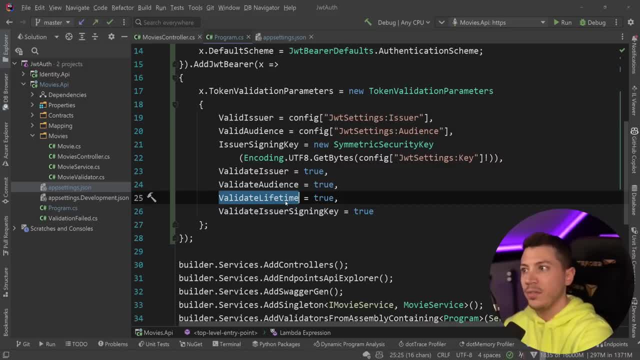 this kind of coin so that it is in effect because you can actually and load these things from somewhere that is designed to store and load these things. and then we say that we bring something for future funds祂c to load these things. and then we say that we bring something for future funds�mdk OFF, doing this it takes a little bit more time. the token so that it is in effect because you can expected aoksaj. 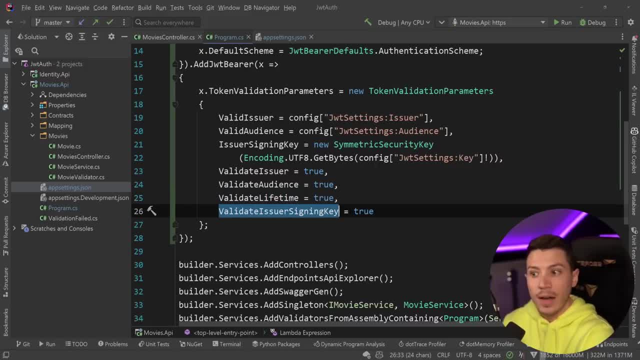 all of these things have to be specified as true, and also that you have to validate the issue assigning key, because that's, ultimately, what makes the jot so powerful: the fact that it is this stateless construct that all you need to do is validate the signature and then the rest is valid. 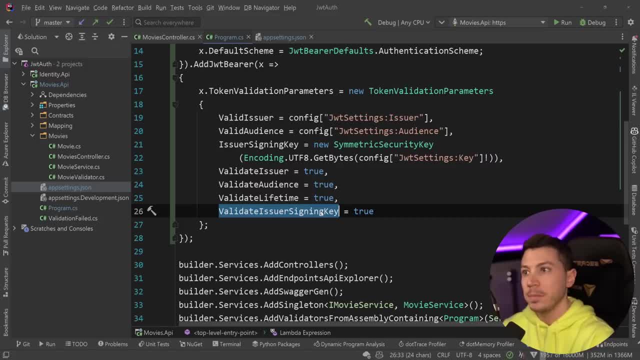 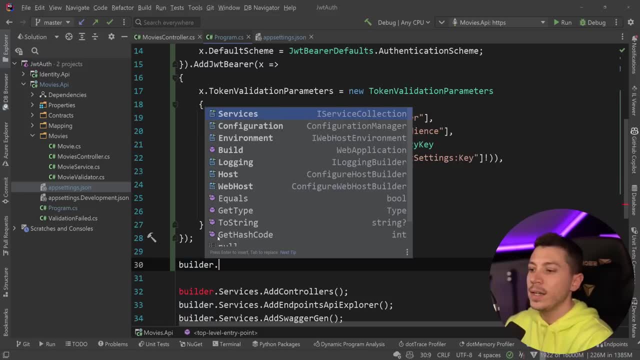 and true, because if the signature is valid, then the rest of the thing must be, because for the hash to be valid, the payload and the header have to also be valid. so this is everything we need, and then the next thing we need is the add authorization call. so i'm going to add it as it is. 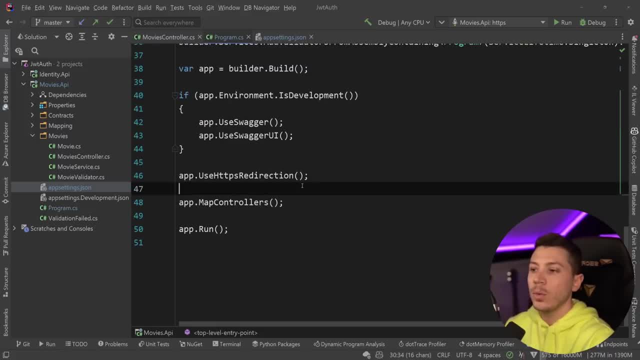 bare bones, nothing in it. and then i'm going to go all the way down to the middleware area and after the https redirection and before the map controllers, i'm going to say use authentication and then app dot use authorization. now remember that sequence in middleware actually matters. so authentication. 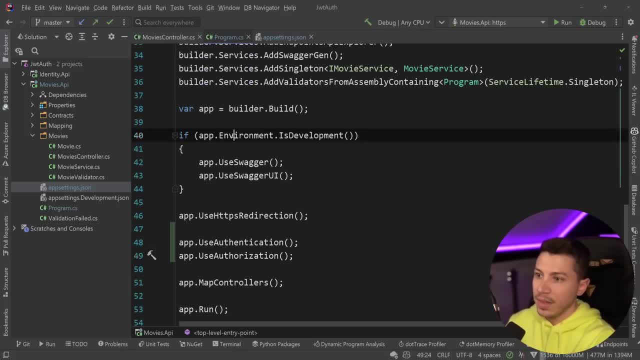 happens. first, authorization second, and then controllers, meaning that everything above it are not part of authentication, authentication, authorization. so be very careful now. actually, in terms of authentication, that is it. obviously. if i just leave my controller as it is and i go and i run it, nothing really will happen. 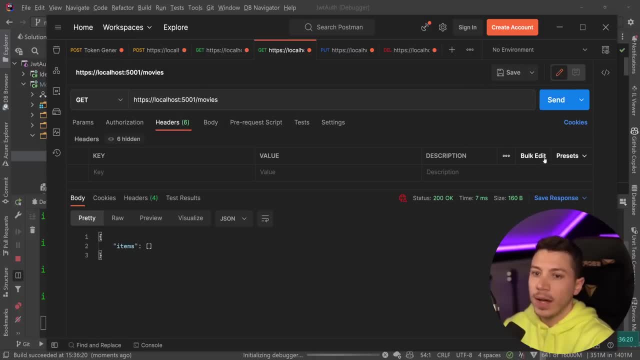 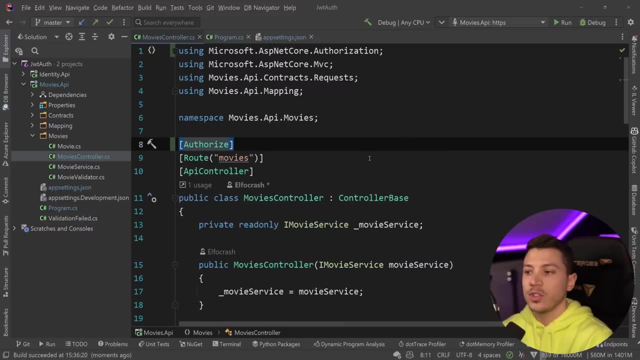 i will still be able to get all my movies in the database. now i have nothing, of course, but nothing really blocks me from getting them. but if i now go in the controller and i say that authorize the users trying to access this controller, and i try to run it again, then i'm going to get a 401. 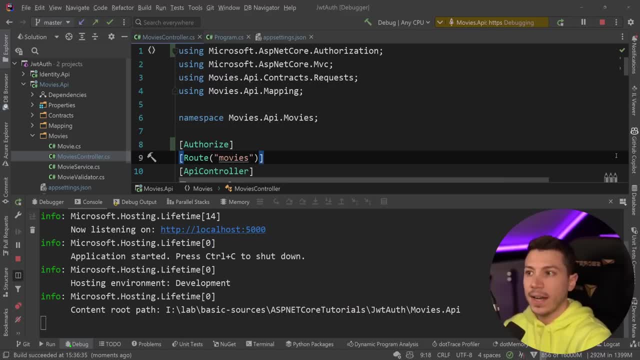 unauthorized because nothing can authenticate me or authorize me to see if i can actually use this controller, and i try to run it again, then i'm going to get a 401- unauthorized because nothing can authenticate me or authorize me to see if i can actually use this api. so how do we pass a json web? 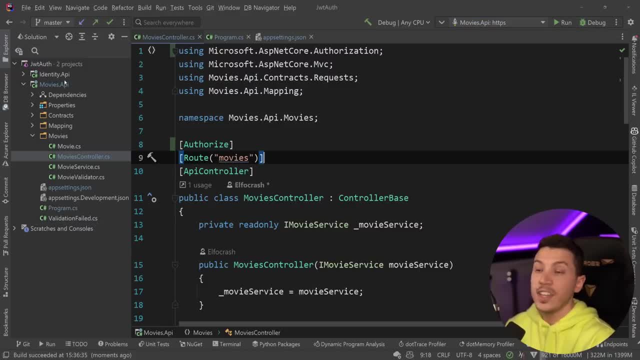 this api. so how do we pass a json web, this api? so how do we pass a json web token to validate that we can actually token to validate that we can actually token to validate that we can actually access it? well, first we create it and i access it. well, first we create it and i. 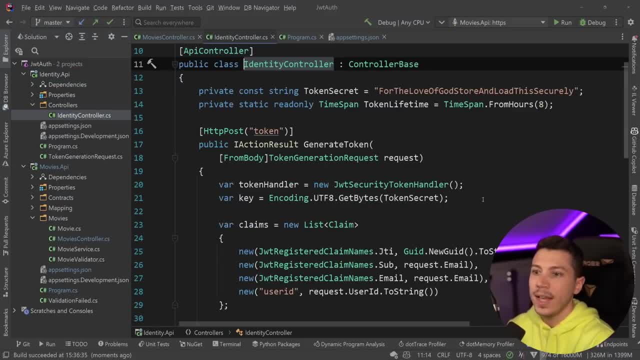 access it. well, first we create it, and i have a helper identity api here that knows. have a helper identity api here that knows. have a helper identity api here that knows how to create a token. it uses the same. how to create a token: it uses the same. 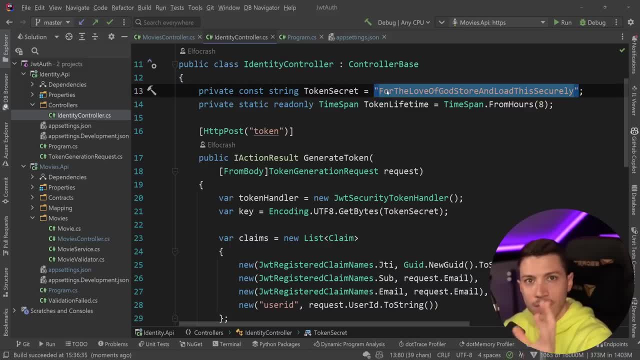 how to create a token. it uses the same key which, again, you don't want to store, key which, again, you don't want to store, key which, again, you don't want to store here as a constant, like jesus, just store here as a constant, like jesus, just store. 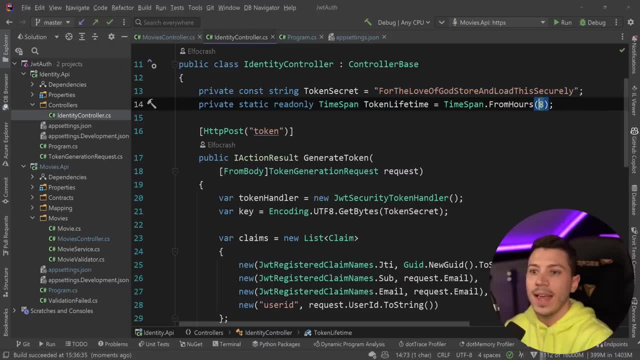 here as a constant, like jesus, just store it somewhere securely. and we're going it somewhere securely. and we're going it somewhere securely and we're going to create a token that lasts for eight. to create a token that lasts for eight. to create a token that lasts for eight hours. this is way too long, usually for 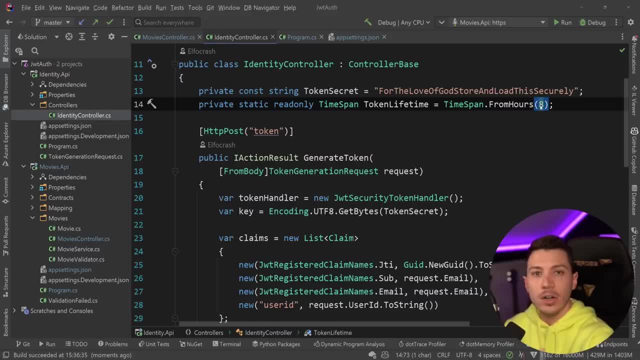 hours. this is way too long usually for hours. this is way too long usually for json web tokens. they're way more json web tokens. they're way more json web tokens. they're way more short-lived and then recreated. and if short-lived and then recreated, and if 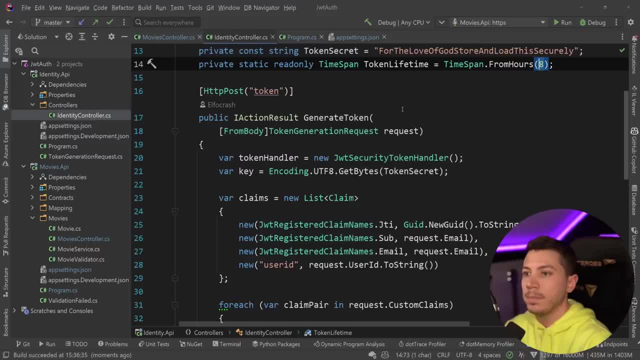 short-lived and then recreated. and if you want to see a video on refreshing, you want to see a video on refreshing. you want to see a video on refreshing tokens. leave a comment down below as tokens. leave a comment down below as tokens. leave a comment down below as well. but then this is the process i can. 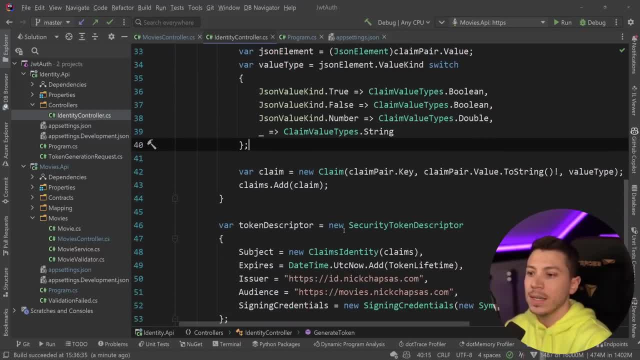 well, but then this is the process i can well, but then this is the process i can follow to generate adjacent web token. follow to generate adjacent web token. follow to generate adjacent web token with all of my custom claims over here, with all of my custom claims over here. 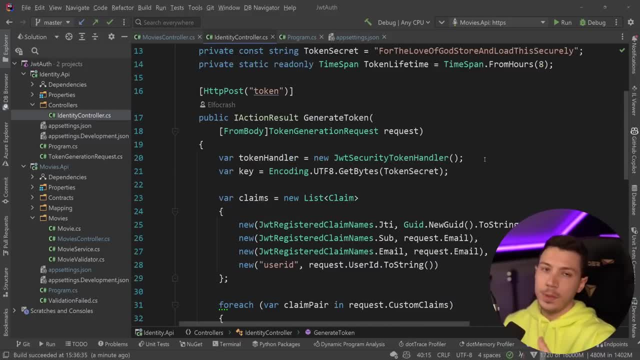 with all of my custom claims over here. you can just grab this and use it for. you can just grab this and use it for. you can just grab this and use it for your own purposes, now, in reality. you, your own purposes now, in reality. you, your own purposes now, in reality. you will be using something like identity. 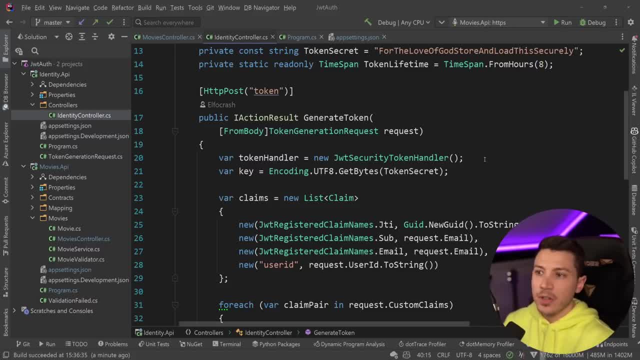 will be using something like identity, will be using something like identity server or octa or auth0 or some service server or octa or auth0 or some service server or octa or auth0 or some service dedicated to creating these types of, dedicated to creating these types of. 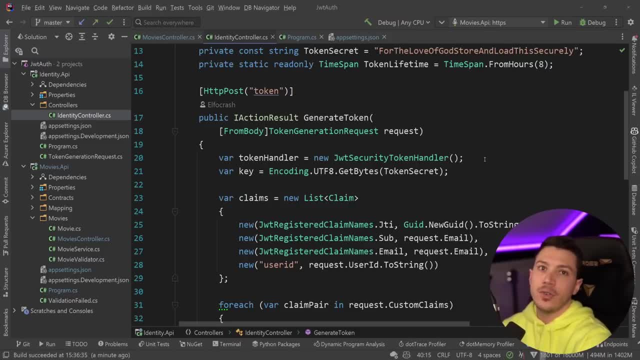 dedicated to creating these types of things in specific flows. but because things in specific flows, but because things in specific flows, but because what these services ultimately generate, what these services ultimately generate, what these services ultimately generate, is adjacent web token we're just going, is adjacent web token, we're just going. 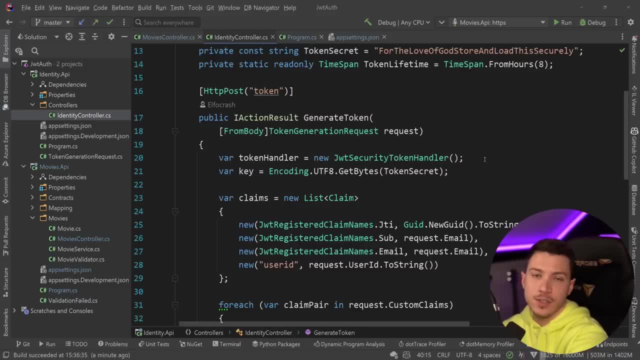 is adjacent web token. we're just going to focus on the implementation side of, to focus on the implementation side of, to focus on the implementation side of things. we're not going to focus on the things. we're not going to focus on the things. we're not going to focus on the creation side of things. so we're just 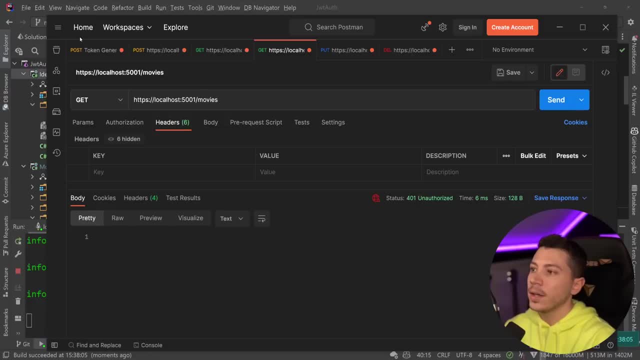 creation side of things. so we're just creation side of things. so we're just going to use this helper service. i'm just going to use this helper service. i'm just going to use this helper service. i'm just going to run it and go back to postman. 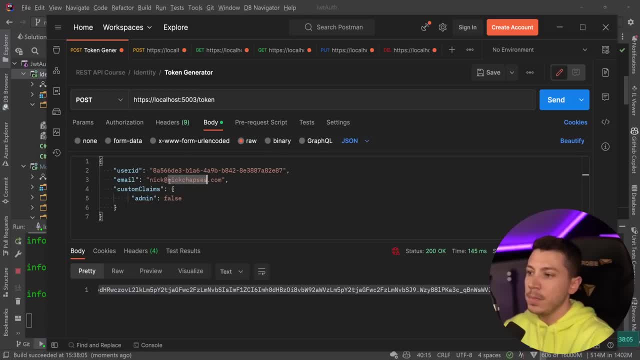 going to run it and go back to postman, going to run it and go back to postman and i'm just going to say that, hey, this. and i'm just going to say that, hey this. and i'm just going to say that, hey, this is me, this is my user id. create a token. 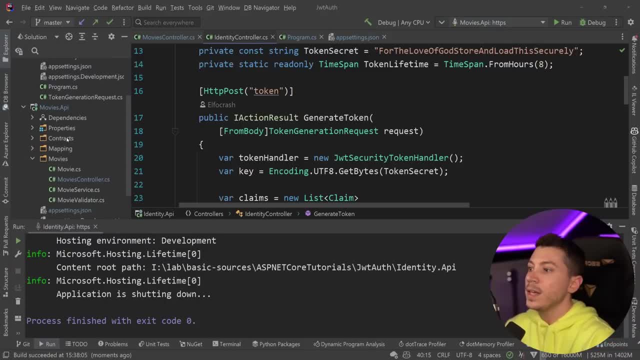 is me. this is my user id. create a token is me. this is my user id. create a token, and i have a token to use it, so i'm, and i have a token to use it, so i'm, and i have a token to use it, so i'm going to stop this api and run the. 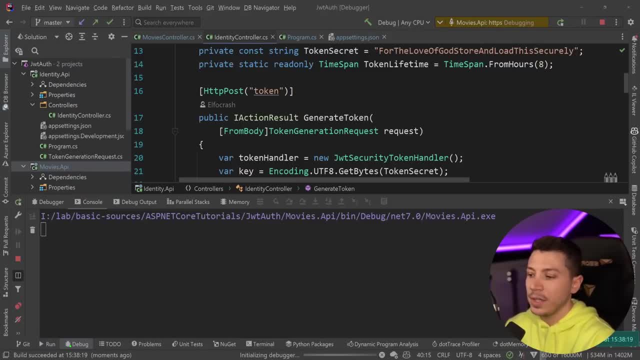 going to stop this api and run the. going to stop this api and run the movies api. remember, we cannot access movies api. remember, we cannot access movies api. remember, we cannot access this because we're not authenticated, but this because we're not authenticated, but this because we're not authenticated. but to say that, hey, it's nick, can i please? 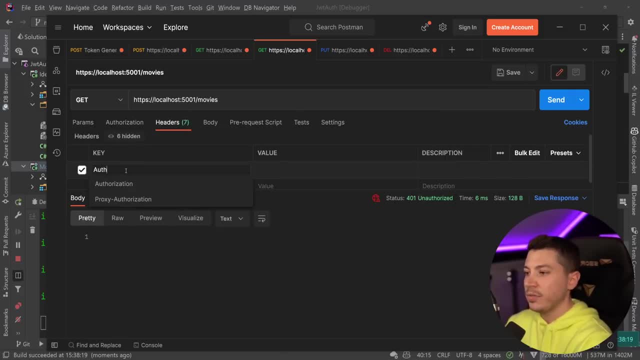 to say that? hey, it's nick. can i please to say that? hey, it's nick. can i please access this? all i'm going to do is go to access this. all i'm going to do is go to access this. all i'm going to do is go to the headers and specify the. 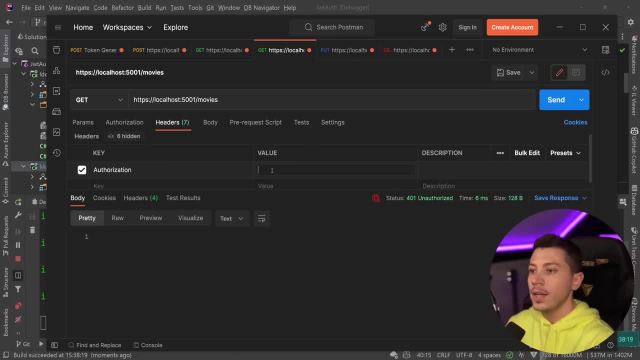 the headers and specify the the headers and specify the authorization header. but it's not just authorization header, but it's not just authorization header, but it's not just pasting the token. you actually have to pasting the token. you actually have to pasting the token. you actually have to say: 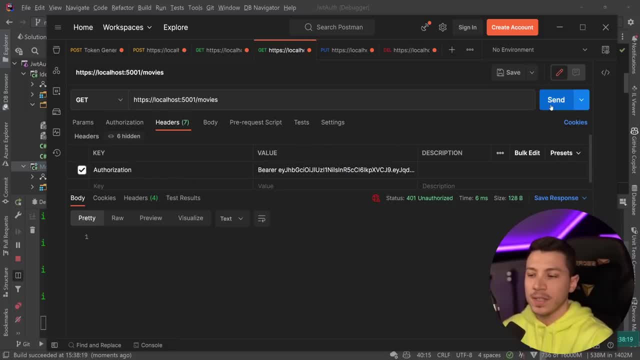 say, say bearer space, and then the token it's bearer space, and then the token it's bearer space, and then the token it's just the way of passing down a bearer, just the way of passing down a bearer, just the way of passing down a bearer token. and now, if i have that, i can go. 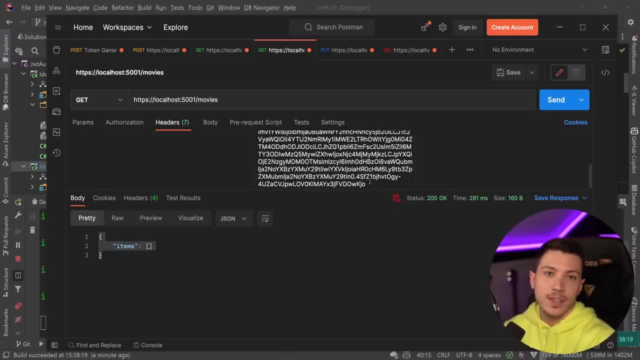 token, and now if i have that, i can go token, and now if i have that, i can go ahead and i can get the item. so i am ahead and i can get the item. so i am ahead and i can get the item. so i am authenticate. and in this case, 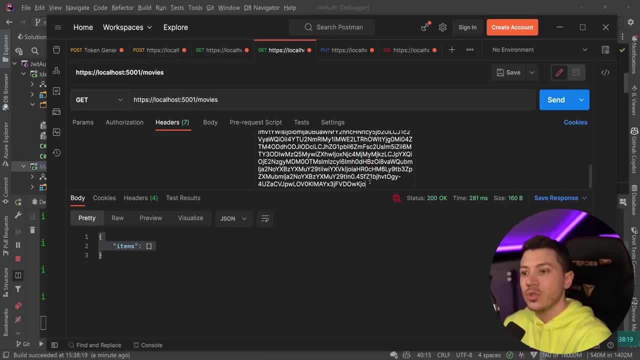 authenticate and in this case, authenticate and in this case, authorized as well, because we don't authorized as well, because we don't authorized as well, because we don't really check for anything. if the really check for anything, if the really check for anything, if the signature was different, if, in the end, i signature was different. if, in the end, i signature was different. if in the end i have a zero, not an o, then i'm going to have a zero, not an o. then i'm going to have a zero, not an o, then i'm going to get an unauthorized because the 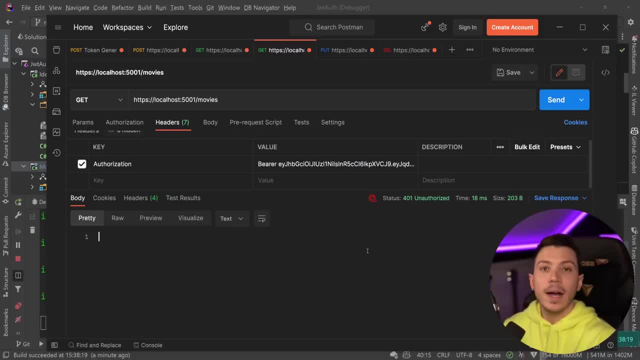 get an unauthorized because the get an unauthorized because the signature is invalid. if this thing was signature is invalid, if this thing was signature is invalid, if this thing was expired, then i would get an expired. then i would get an expired, then i would get an unauthorized as well, but in this case i 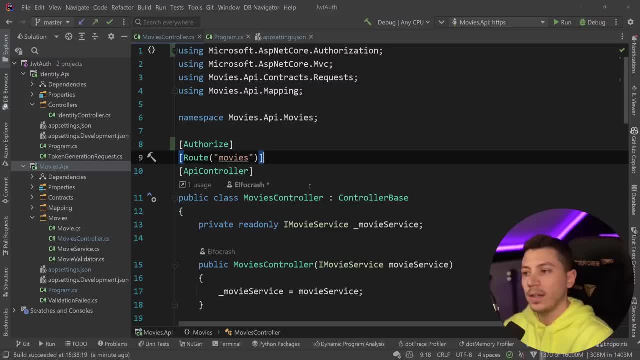 unauthorized as well, but in this case i unauthorized as well, but in this case i have a good token. so nothing really have a good token. so nothing really have a good token. so nothing really breaks. everything just works, now, let's breaks. everything just works now, let's. 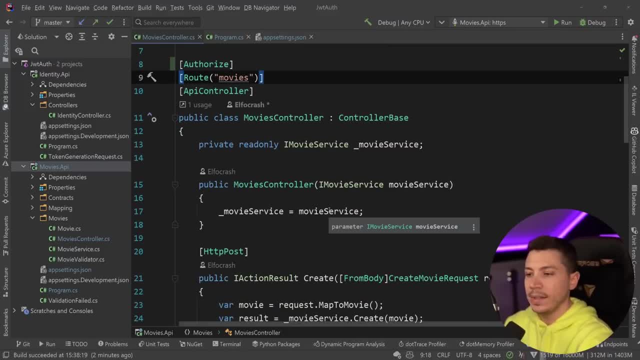 breaks. everything just works. now let's talk about a very important thing. what talk about a very important thing? what talk about a very important thing? what if i want my create, update and delete, if i want my create, update and delete, if i want my create, update and delete to be authenticated and authorized, but to be authenticated and authorized, but to be authenticated and authorized, but my get doesn't really matter. i want my get doesn't really matter. i want my get doesn't really matter. i want everyone to be able to access it. you, everyone to be able to access it, you. 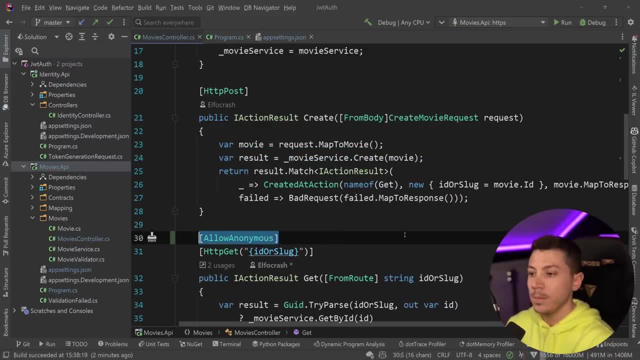 everyone to be able to access it. you have two approaches here. you can either have two approaches here. you can either have two approaches here. you can either say allow anonymous here and this allow- say allow anonymous here and this allow- say allow anonymous here and this allow anonymous attribute will override the. 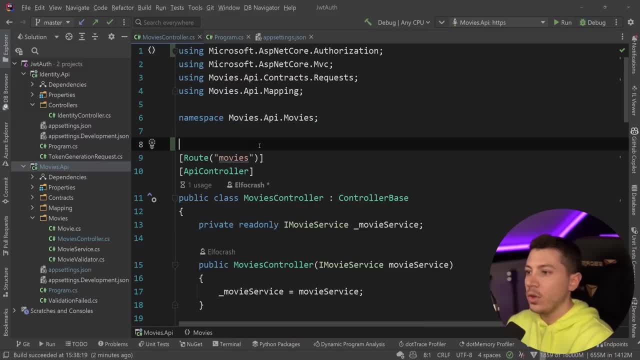 anonymous attribute will override the anonymous attribute will override the overarching controller based behavior, or overarching controller based behavior or overarching controller based behavior. or we can just take the authorized from the, we can just take the authorized from the. we can just take the authorized from the controller and we can paste it on each. 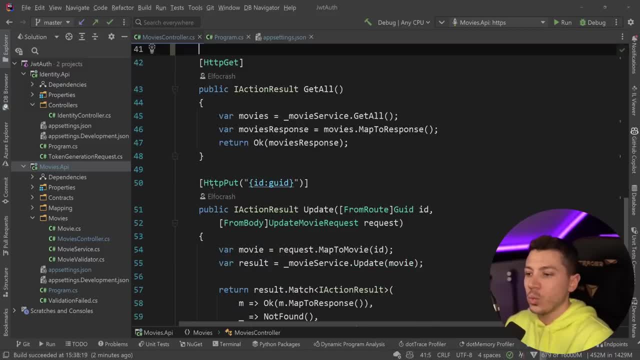 controller and we can paste it on each controller. and we can paste it on each individual thing we want. authorized you, individual thing we want. authorized you, individual thing we want. authorized you can ultimately choose which one you want, can ultimately choose which one you want, can ultimately choose which one you want to use in general, having it on a pair. 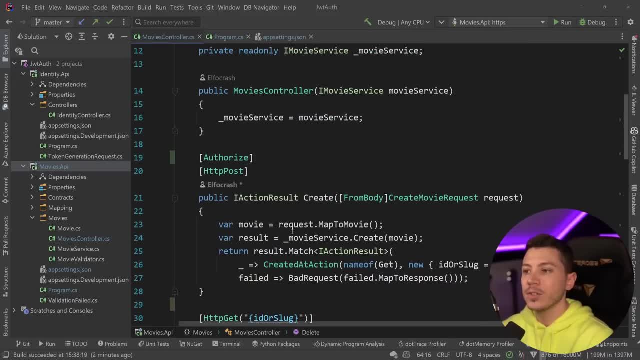 to use in general. having it on a pair to use in general, having it on a pair action basis is actually more used. mainly action basis is actually more used. mainly action basis is actually more used mainly because it allows you to specify. because it allows you to specify, 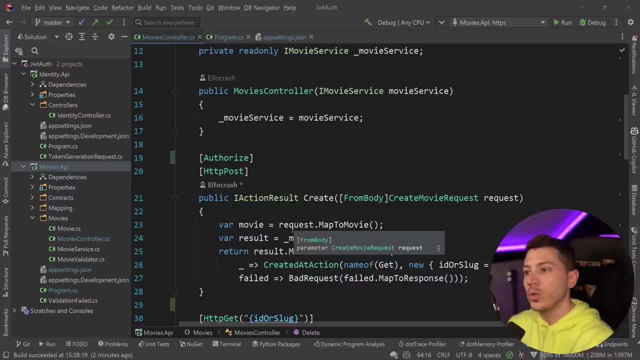 because it allows you to specify different things on the action itself and different things on the action itself and different things on the action itself. and this is actually where authorization, this is actually where authorization, this is actually where authorization comes in, or the process of validating comes in, or the process of validating. 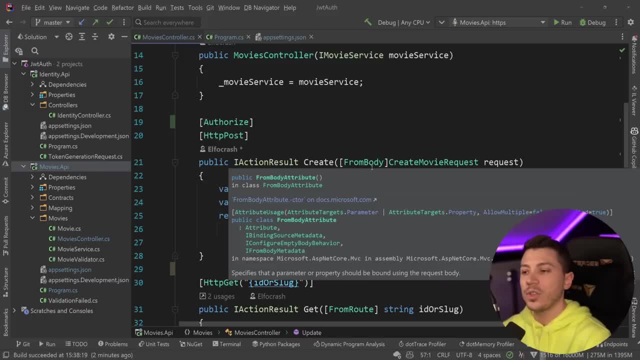 comes in, or the process of validating that someone can do what they claim to, that someone can do what they claim to, that someone can do what they claim to do, for example. i want everyone who's do. for example, i want everyone who's do. for example, i want everyone who's authenticated to create and update a. 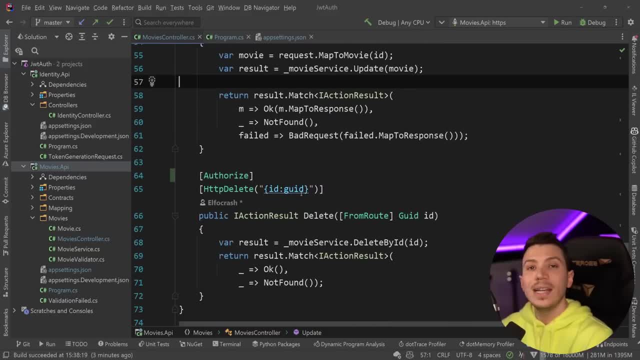 authenticated to create and update a. authenticated to create and update a movie, but i want only admins or movie. but i want only admins or movie, but i want only admins or administrators to delete a movie. how do i administrators to delete a movie? how do i administrators to delete a movie? how do i do that? well, there's a few ways, but the 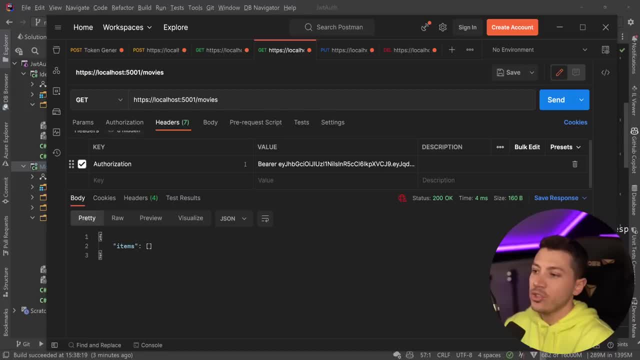 do that. well, there's a few ways, but the do that. well, there's a few ways, but the simplest one is by using a claim. so, in simplest one is by using a claim. so in simplest one is by using a claim. so in that json web token, if you remember what, 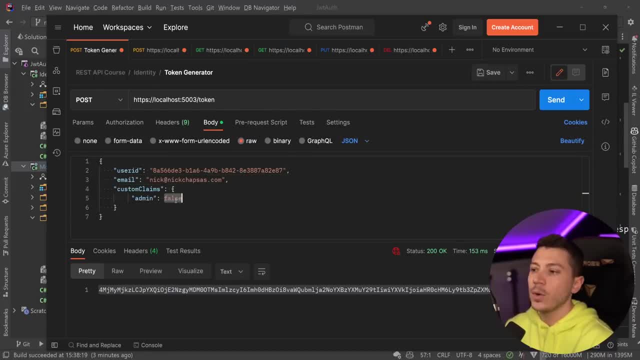 that json web token. if you remember what that json web token, if you remember what i said in a custom claim, is that an i said in a custom claim is that an i said in a custom claim is that an admin is false. now, usually when someone. admin is false, now usually when someone. 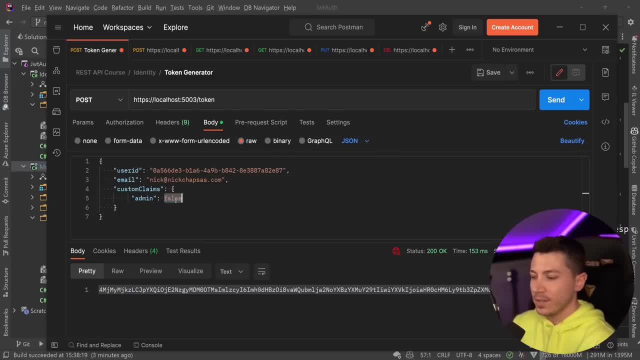 admin is false. now, usually when someone is not something you wouldn't have it in, is not something you wouldn't have it in, is not something you wouldn't have it in the token, you would just not have the the token- you would just not have the the token, you would just not have the claim at all. the absence of a claim. 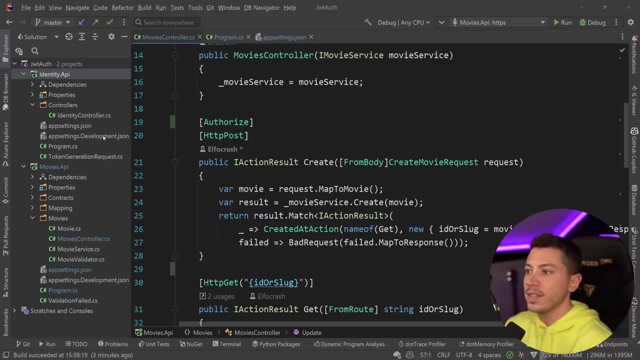 claim at all the absence of a claim. claim at all. the absence of a claim means that that user is not something, means that that user is not something, means that that user is not something. but if i just run this api again and i, but if i just run this api again and i, 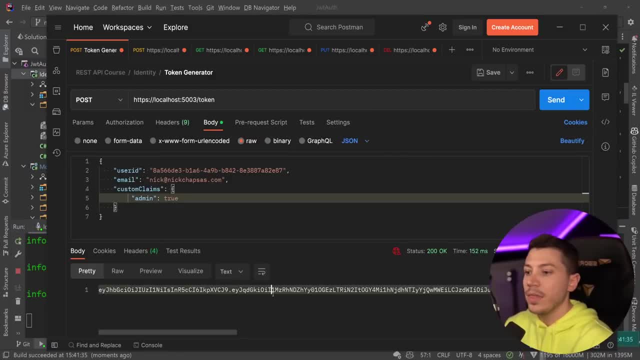 but if i just run this api again and i regenerate this token and i say that, regenerate this token. and i say that, regenerate this token, and i say that, yes, this is actually an admin, then i, yes, this is actually an admin, then i, yes, this is actually an admin, then i have a token of someone who is an admin. 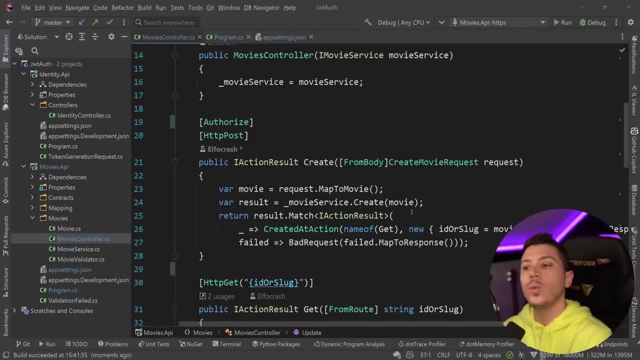 have a token of someone who is an admin. have a token of someone who is an admin and can delete on top of create and and can delete on top of create and and can delete on top of create and update now. how do we implement that well? update now. how do we implement that well? 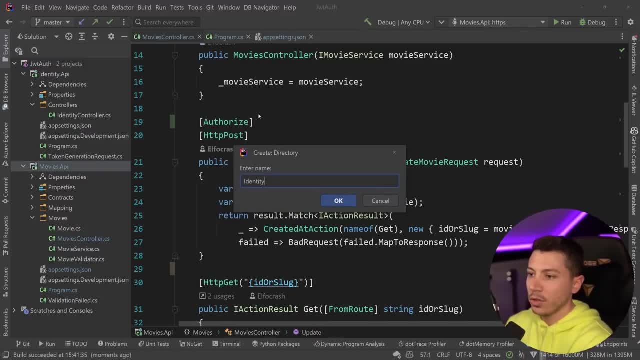 update. now, how do we implement that? well, what we're going to do is create an. what we're going to do is create an. what we're going to do is create an identity folder over here, and i'm just: identity folder over here, and i'm just. 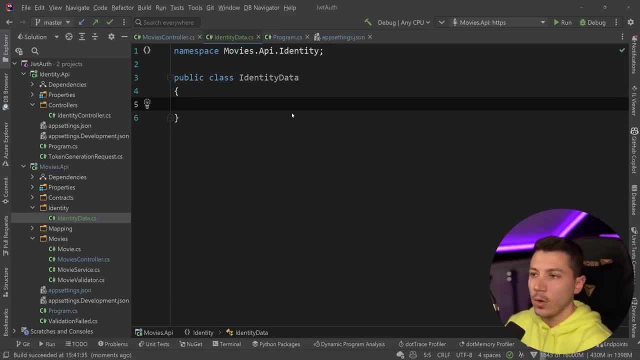 identity folder over here and i'm just gonna create a new class called identity, gonna create a new class called identity, gonna create a new class called identity. that is the admin user policy. now these. that is the admin user policy. now these. that is the admin user policy. now, these things are different. the claim is a. 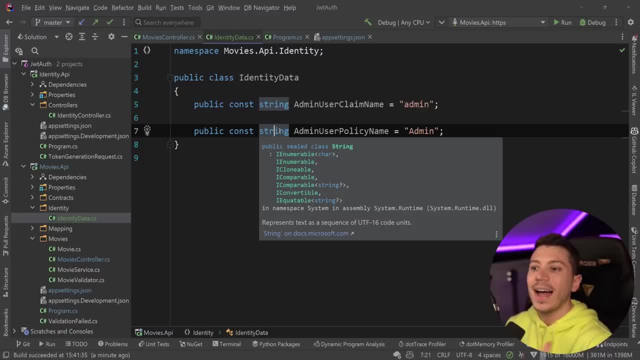 things are different. the claim is a. things are different. the claim is a gestion web token concern. the policy is gestion web token concern. the policy is gestion web token concern. the policy is an application concern. i can define my an application concern. i can define my an application concern. i can define my own policies based on claims or other. 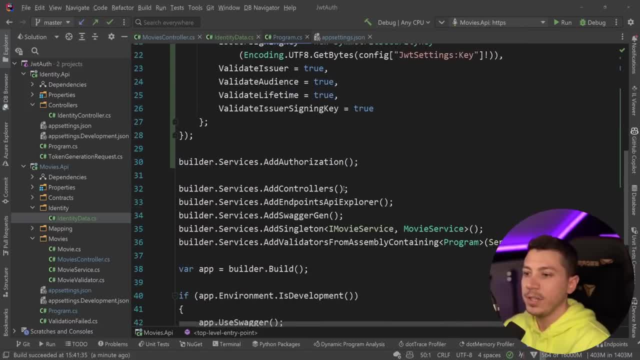 own policies based on claims or other own policies based on claims or other things to create a policy. all i'm going things to create a policy. all i'm going things to create a policy. all i'm going to do is go all the way up here to add: 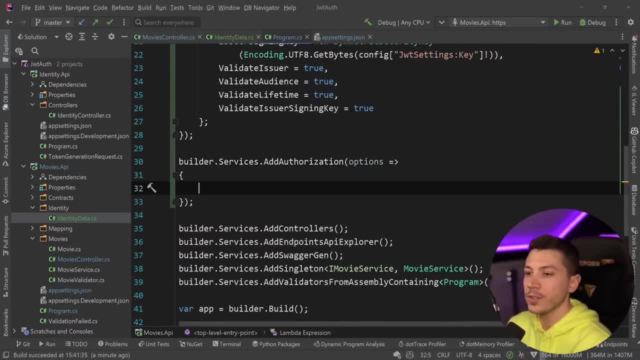 to do is go all the way up here to add. to do is go all the way up here to add authorization and i'm going to say authorization and i'm going to say authorization and i'm going to say authorization options and say options: authorization options and say options. 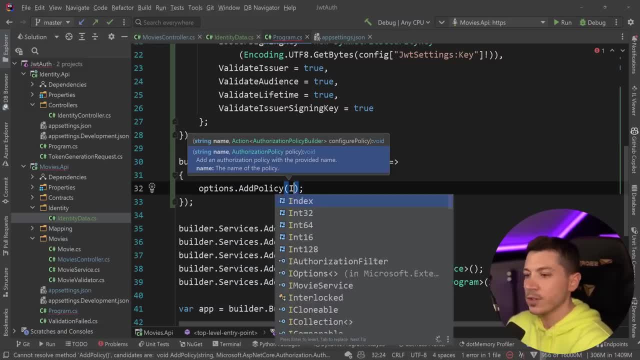 authorization options and say options, dot add policy, and i can create my own dot add policy. and i can create my own dot add policy and i can create my own policy using a name. so i'm gonna say policy using a name. so i'm gonna say policy using a name. so i'm gonna say identity data equals admin user policy. 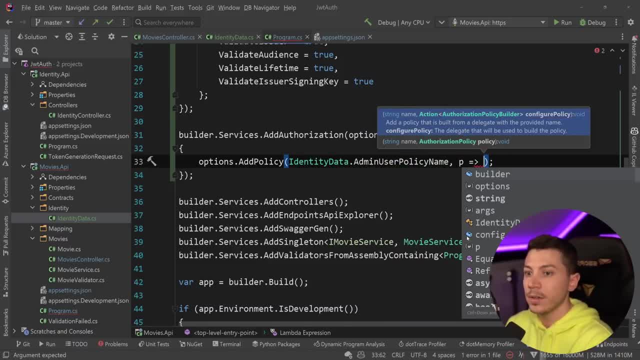 identity data equals admin user policy. identity data equals admin user policy name. and then what do i want? i want a name. and then what do i want? i want a name. and then what do i want? i want a policy using this policy builder, that policy using this policy builder, that. 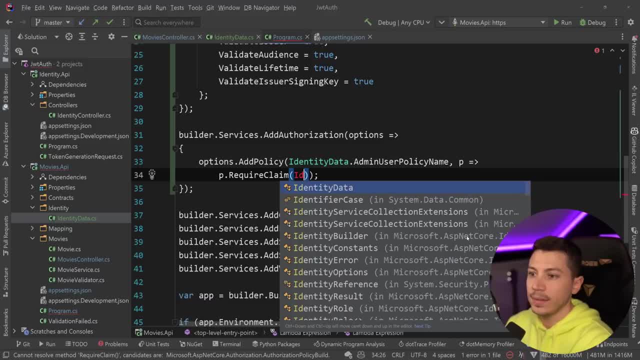 policy using this policy builder. that requires a claim and the claim i want requires a claim and the claim i want requires a claim. and the claim i want is in identity data dot admin user claim is in identity data dot admin user claim. is in identity data dot admin user claim name and the value i want for this. 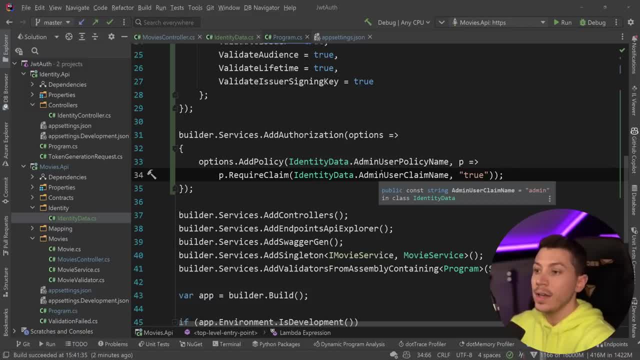 name and the value i want for this name and the value i want for this policy is true. so now i have my policy policy is true. so now i have my policy policy is true. so now i have my policy registered. it's not used anywhere by registered. it's not used anywhere by. 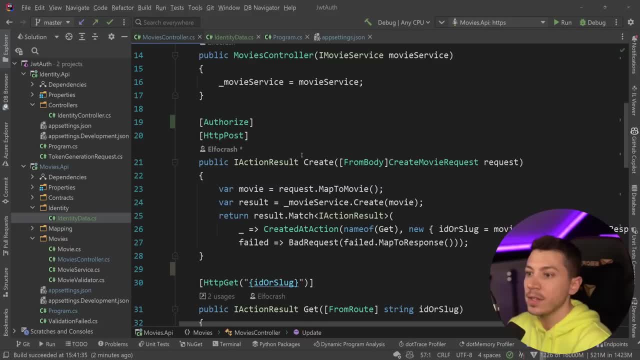 registered. it's not used anywhere by default. we just have it now in the default. we just have it now in the default. we just have it now in the system. we can go ahead and just copy system. we can go ahead and just copy system. we can go ahead and just copy this and we can say that you know what? this and we can say that you know what this and we can say that you know what create and update doesn't really need this. and we can say that you know what create and update doesn't really need this, and we can say that you know what create and update doesn't really need anything. i'll go all the way to delete over. 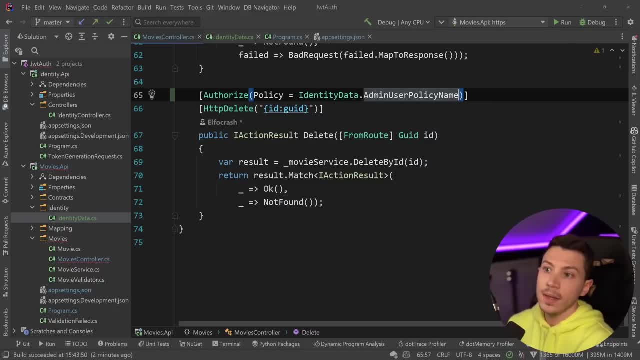 anything. i'll go all the way to delete over anything. i'll go all the way to delete over here and say that actually i want this here, and say that actually i want this here. and say that actually i want this policy to be identity data dot admin. 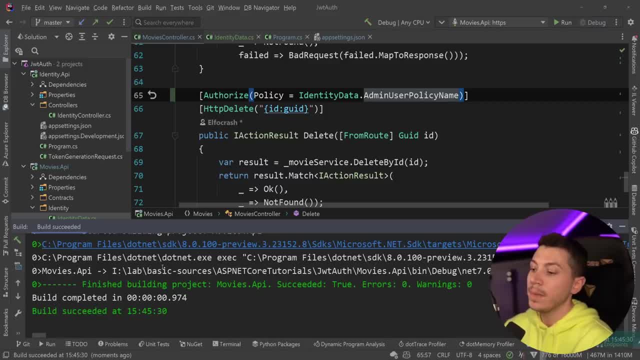 policy to be identity data dot. admin policy. to be identity data dot. admin. user policy. to delete and move in the user policy. to delete and move in the user policy. to delete and move in the system. so i'm going to run this and i'm system. so i'm going to run this and i'm 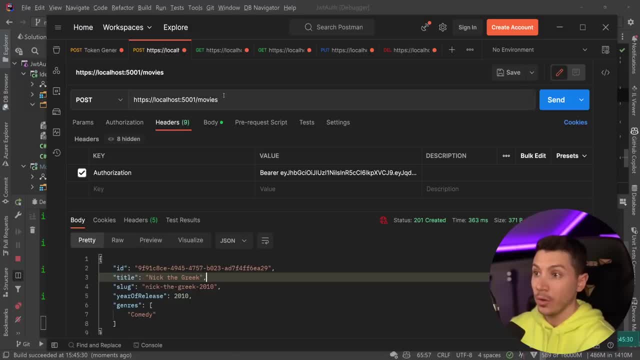 system. so i'm going to run this and i'm going to use the previous token. i have going to use the previous token. i have going to use the previous token. i have that has admin as false. so if i try to, that has admin as false. so if i try to, 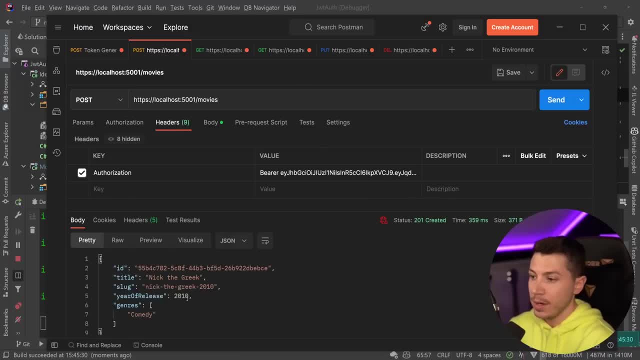 that has admin as false. so if i try to create a movie using that old token, the create a movie using that old token, the create a movie using that old token, the non-admin token, then i can and i get my non-admin token, then i can and i get my. 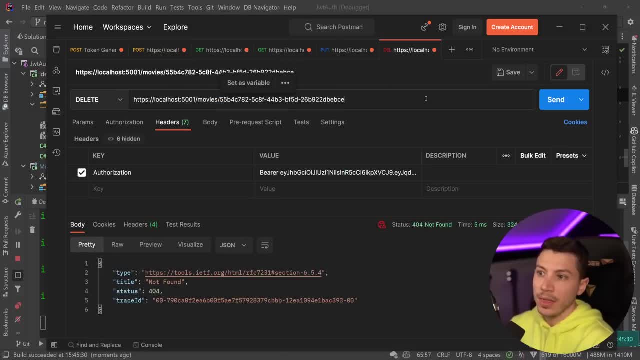 non-admin token, then i can and i get my movie. but if i go to delete over here to movie, but if i go to delete over here to movie, but if i go to delete over here to delete that movie without being an admin, delete that movie without being an admin. 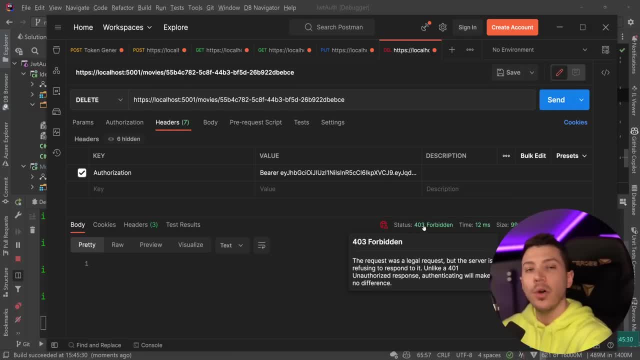 delete that movie without being an admin. what i'm going to get is 403 forbidden. what i'm going to get is 403 forbidden. what i'm going to get is 403 forbidden, not 401 unauthorized forbidden. you're not 401 unauthorized forbidden, you're. 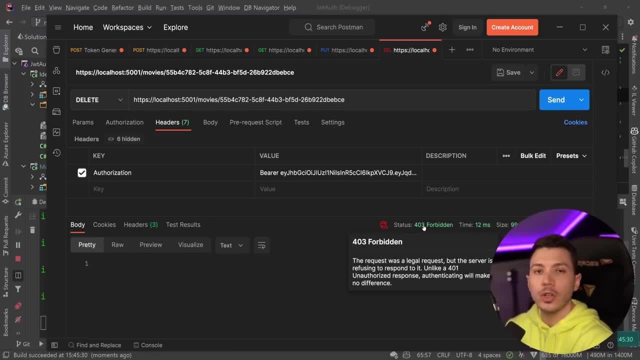 not 401 unauthorized forbidden. you're forbidden to make this action and that. forbidden to make this action and that forbidden to make this action. and that is because i just don't match the, is because i just don't match the, is because i just don't match the profile that the policy requires me to. 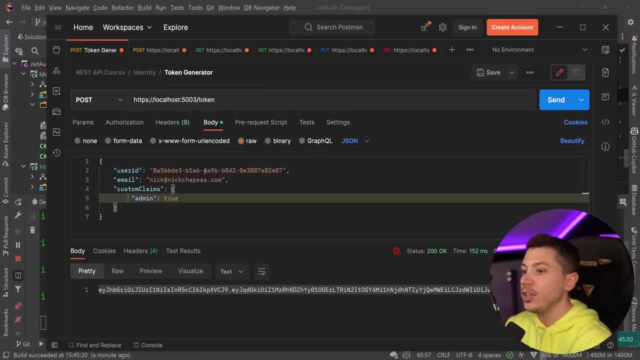 profile that the policy requires me to profile, that the policy requires me to have, which is having the claim as true. have, which is having the claim as true. have, which is having the claim as true. now, if i go and i use this new token. now, if i go and i use this new token. 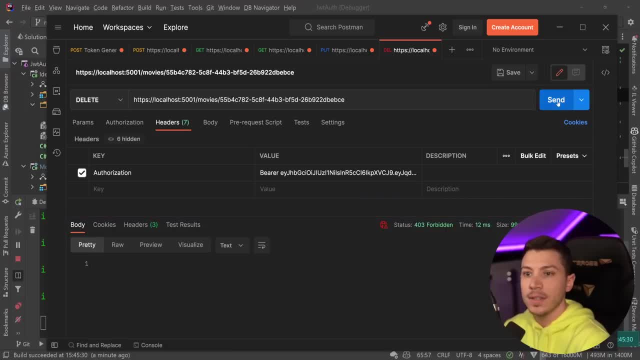 now, if i go and i use this new token over here, which is an admin, then i can over here, which is an admin, then i can over here, which is an admin, then i can go here replace this send, and now it is. go here, replace this send, and now it is. 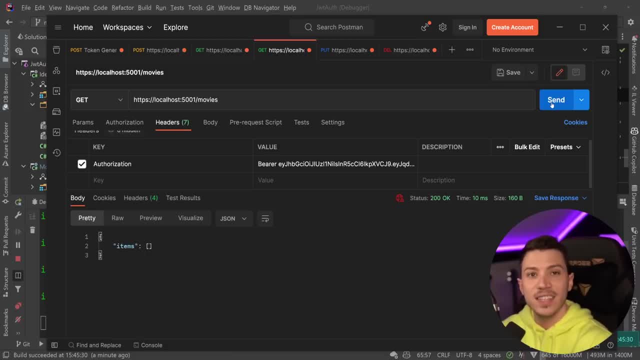 go here, replace this send. and now it is deleted and it no longer exists in the deleted. and it no longer exists in the deleted and it no longer exists in the system. and that is it now you can go. system. and that is it, now you can go. 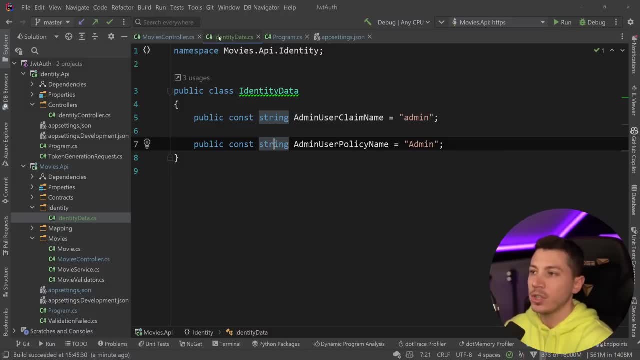 system and that is it. now you can go even deeper and have multiple policies even deeper and have multiple policies even deeper and have multiple policies and mix and match on different things and mix and match on different things and mix and match on different things and customer sessions, but this is the. 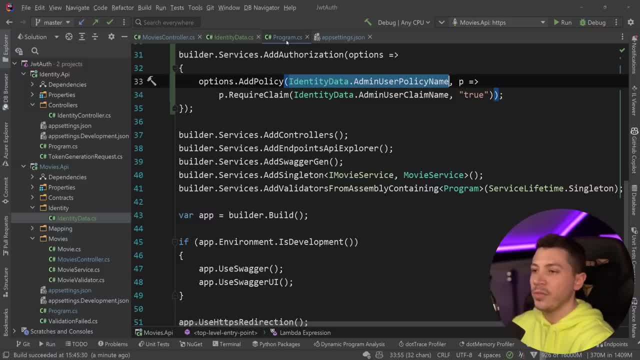 and customer sessions, but this is the. and customer sessions, but this is the most basic way of making a policy, most basic way of making a policy, most basic way of making a policy. however, some people prefer to validate. however, some people prefer to validate. however, some people prefer to validate based on a single claim, without using a 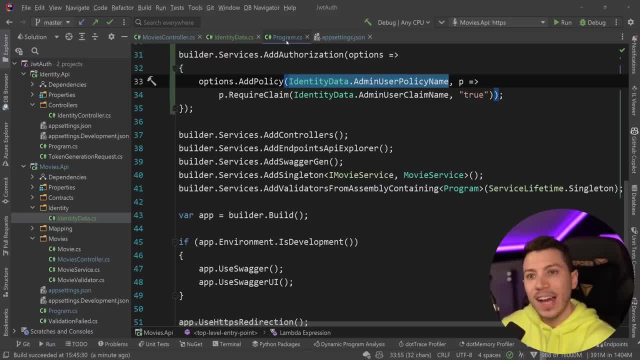 based on a single claim without using a. based on a single claim without using a policy, and one of the preferred ways is policy. and one of the preferred ways is policy, and one of the preferred ways is to actually create a custom attribute, to actually create a custom attribute. 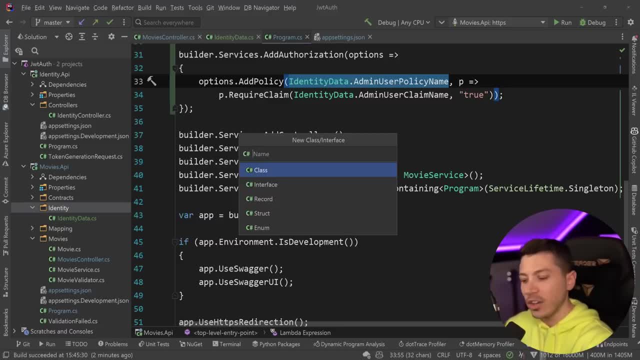 to actually create a custom attribute which validates claims. what i'm going to- which validates claims, what i'm going to which validates claims. what i'm going to do is create a new attribute called do is create a new attribute called do is create a new attribute called requires claim attribute. over here and. 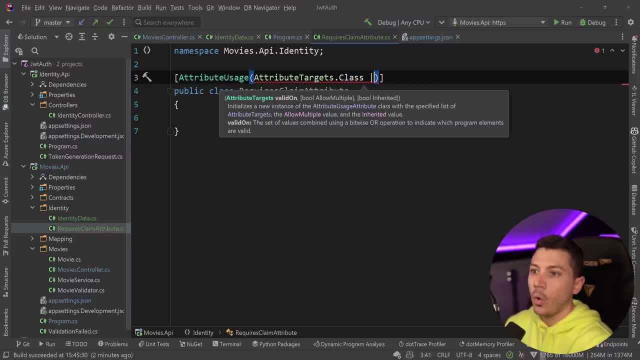 requires claim attribute over here and requires claim attribute over here and i'm going to have that be an attribute. i'm going to have that be an attribute. i'm going to have that be an attribute used on classes or methods, and it's used on classes or methods and it's. 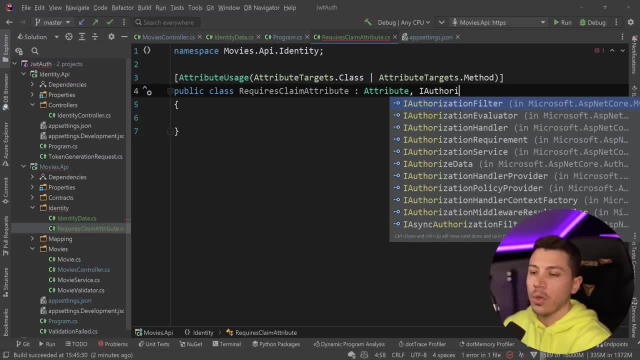 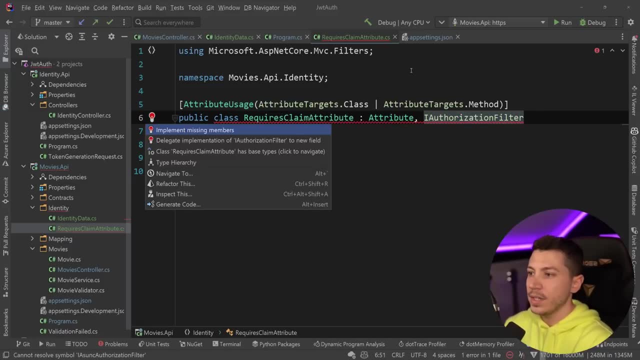 used on classes or methods and it's going to extend application and going to extend application and going to extend application and implement i authorization filter. if you implement i authorization filter, if you implement i authorization filter, if you authorization method, now this is not authorization method, now this is not. 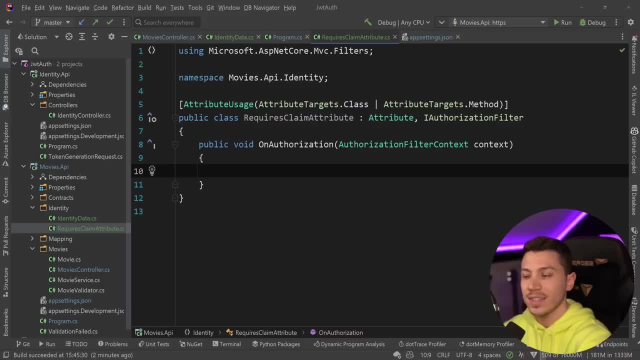 authorization method. now, this is not usable with minimal apis because of how usable with minimal apis, because of how usable with minimal apis, because of how the filtering works there. however, for the filtering works there. however, for the filtering works there. however, for controllers, this does work, if you want. controllers, this does work. if you want controllers, this does work. if you want to have the equivalent of this in, to have the equivalent of this in, to have the equivalent of this in minimal apis, you have to use a minimal minimal apis. you have to use a minimal. 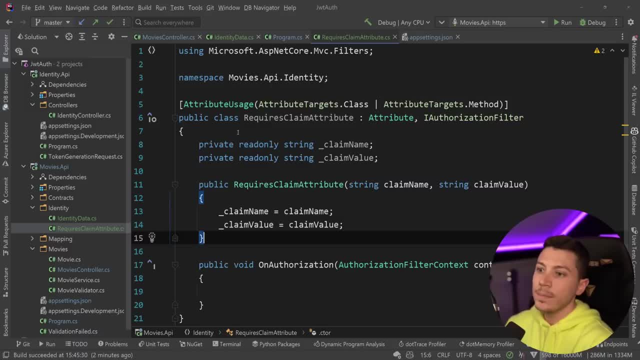 minimal apis. you have to use a minimal apis endpoint filter. and now, here all we apis endpoint filter. and now, here all we apis endpoint filter. and now here, all we need to pass down is a claims name and need to pass down is a claims name, and need to pass down is a claims name and the claims value that we expect, and then 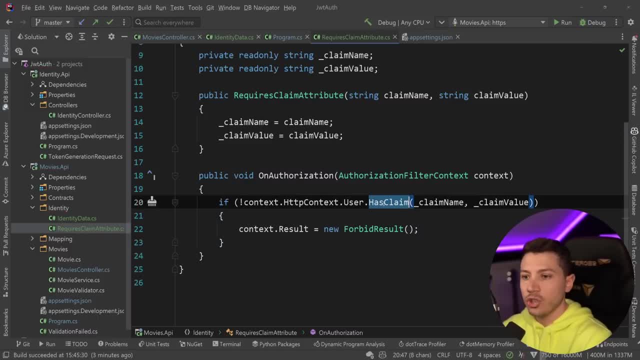 the claims value that we expect, and then the claims value that we expect, and then all we need to say in all authorization, all we need to say in all authorization, all we need to say in all authorization is: hey, if this user doesn't have this is hey if this user doesn't have this. 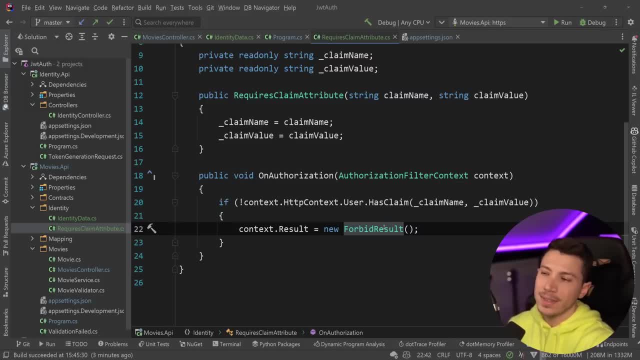 is: hey, if this user doesn't have this claim with this value, then say forbid. or claim with this value, then say forbid. or claim with this value, then say forbid. or unauthorized, depending on how the flow. unauthorized, depending on how the flow. unauthorized, depending on how the flow works in your application. the reason why: 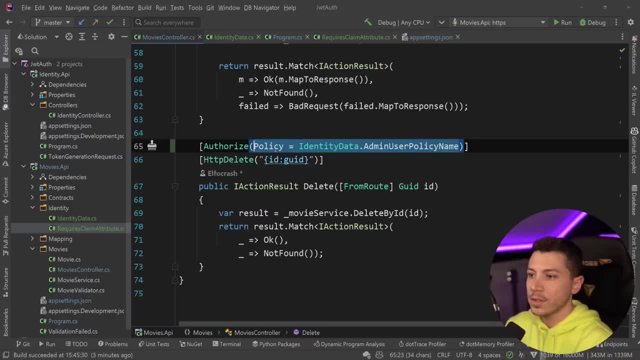 works in your application. the reason why works in your application, the reason why i say that is because in this example i say that is because in this example i say that is because in this example over here, what we're going to say is: over here, what we're going to say is: 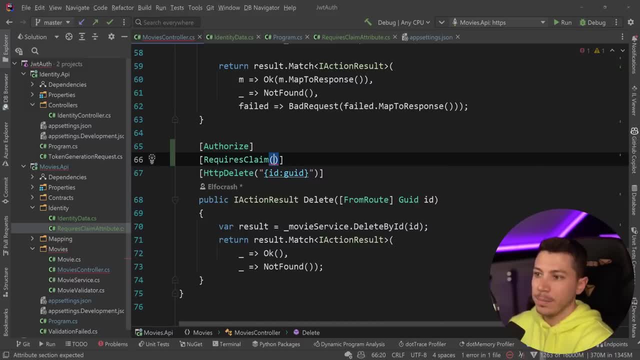 over here. what we're going to say is actually authorized first, and then actually authorized first, and then actually authorized first, and then requires claim second, and all we need requires claim second, and all we need requires claim second, and all we need here is actually the identity data dot. 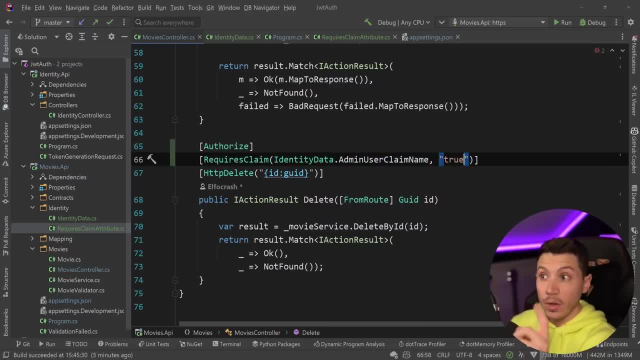 here is actually the identity data dot. here is actually the identity data dot: admin user claim name and the value. admin user claim name and the value. admin user claim name and the value needs to be true and if we do that, i'm needs to be true and if we do that, i'm. 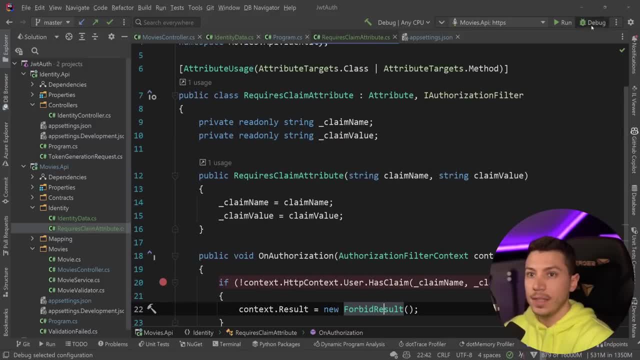 needs to be true. and if we do that, i'm going to put a breakpoint, going to put a breakpoint, going to put a breakpoint in the attribute and then go ahead and in the attribute, and then go ahead and in the attribute, and then go ahead and debug the application. and again the same. 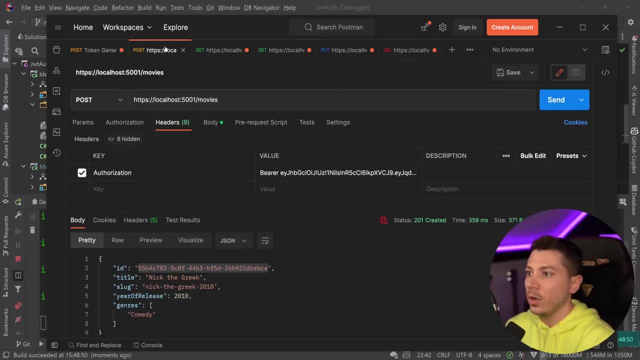 debug the application and again the same. debug the application and again the same way as before. i'm going to revert to way as before. i'm going to revert to way as before. i'm going to revert to the old token. in fact, first i'm going to 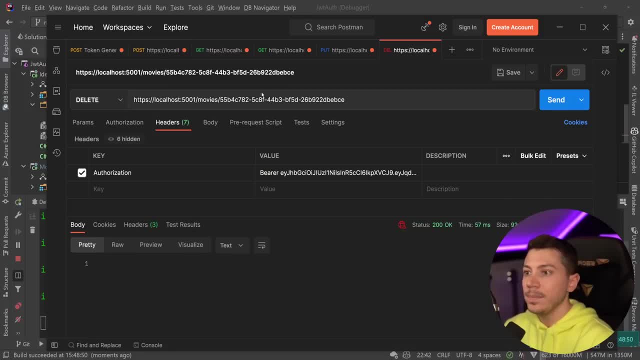 the old token. in fact, first i'm going to the old token. in fact, first i'm going to generate a movie, so the movie is created. generate a movie, so the movie is created. generate a movie, so the movie is created. take that id and then try to delete that. 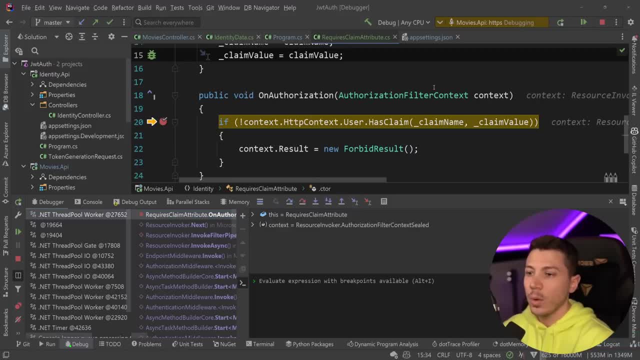 take that id and then try to delete that. take that id and then try to delete that movie with the valid token, and let's see movie with the valid token. and let's see movie with the valid token and let's see what happens. oh, request comes in here we. 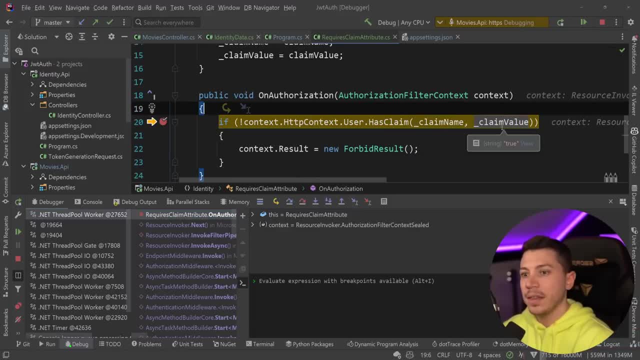 what happens? oh request comes in here. we. what happens, oh request comes in here. we have the context, we have everything and have the context. we have everything and have the context, we have everything. and then the claim name is admin and the. then the claim name is admin and the. 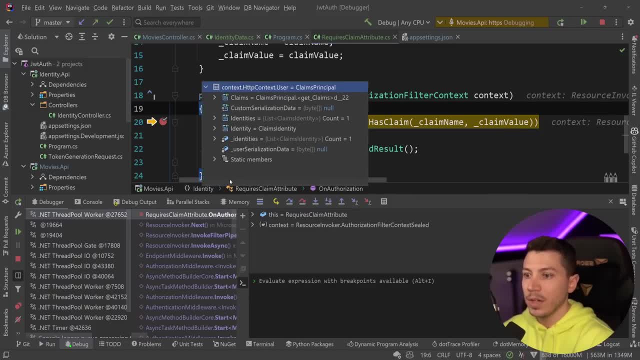 then the claim name is admin and the value we expect is true: is that true? value we expect is true: is that true? value we expect is true, is that true? well, let's see claims principle over. well, let's see claims principle over. well, let's see claims principle over here. and then we have all the claims and 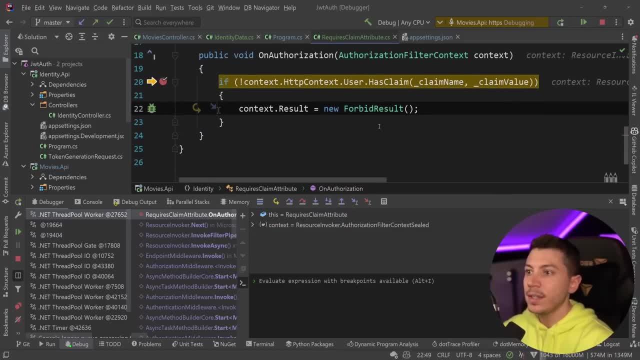 here and then we have all the claims. and here and then we have all the claims and one of them is admin- true, so it will be. one of them is admin true, so it will be one of them is admin true, so it will be validated. so it will have it, it will step. 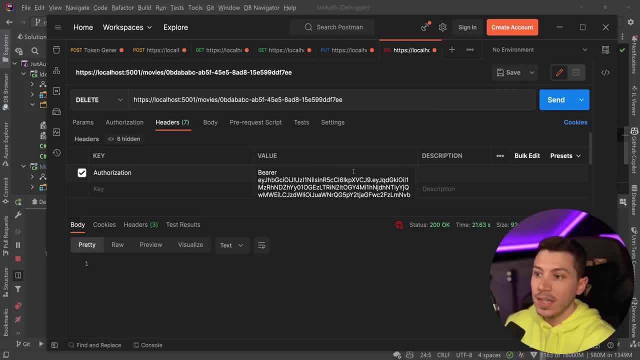 validated, so it will have it. it will step: validated, so it will have it. it will step out of it and the action will in fact out of it, and the action will in fact out of it and the action will in fact happen. okay, if we use the old token and 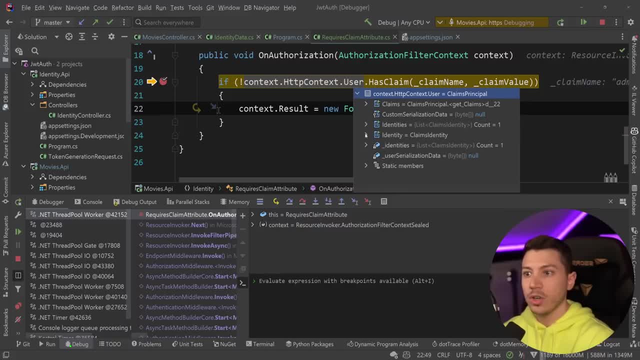 happen okay if we use the old token and happen okay if we use the old token and we try to do the exact same thing. then we try to do the exact same thing, then we try to do the exact same thing. then we come in here but the user claim as: 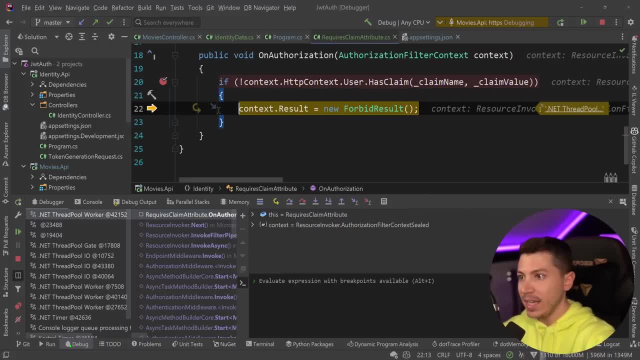 we come in here but the user claim as we come in here. but the user claim, as you can see in the claims is actually you can see in the claims is actually you can see in the claims is actually false. so it's gonna fall in here. say: 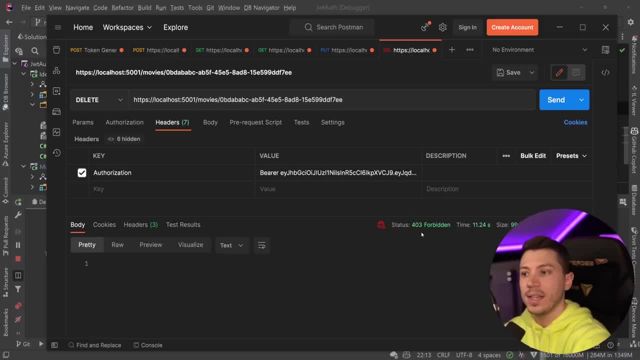 false, so it's gonna fall in here. say false, so it's gonna fall in here: say forbidden and then return 403 forbidden forbidden and then return 403 forbidden forbidden and then return 403 forbidden because we are authenticated but not because we are authenticated but not. 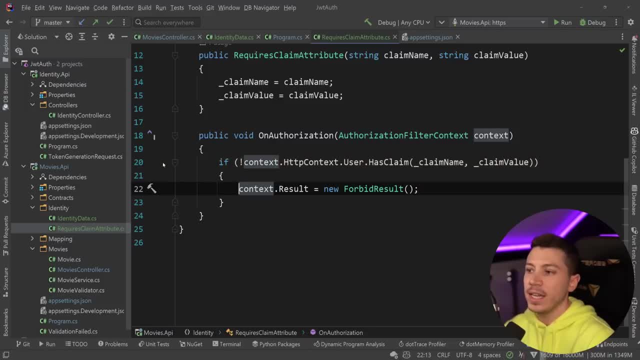 because we are authenticated but not authorized. that's another way you can authorized. that's another way you can authorized. that's another way you can get clever and have a handy approach in get clever and have a handy approach in get clever and have a handy approach in claim based authorization. and you can. 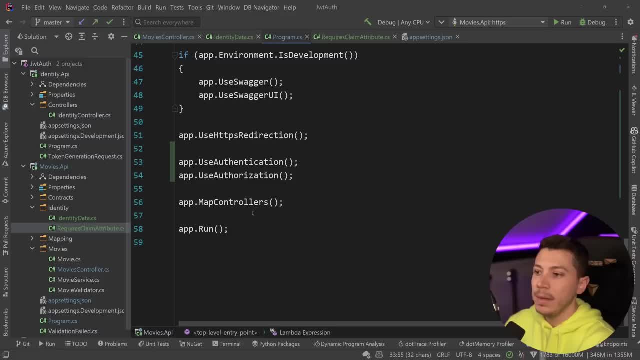 claim based authorization and you can claim based authorization and you can take this in any direction. you want take this in any direction. you want take this in any direction. you want really now, if you were to be using really now, if you were to be using really now, if you were to be using minimal apis, all of those things are. 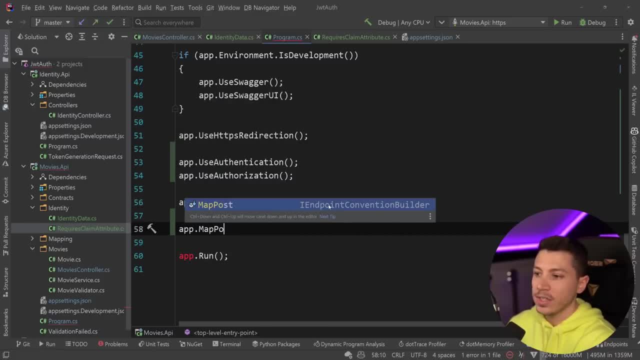 minimal apis. all of those things are minimal apis. all of those things are actually still valid. the difference would actually still valid. the difference would actually still valid. the difference would be that, yes, you can, for example, say map. be that yes, you can, for example, say map. be that, yes, you can, for example, say map post, and let's have a movies endpoint. 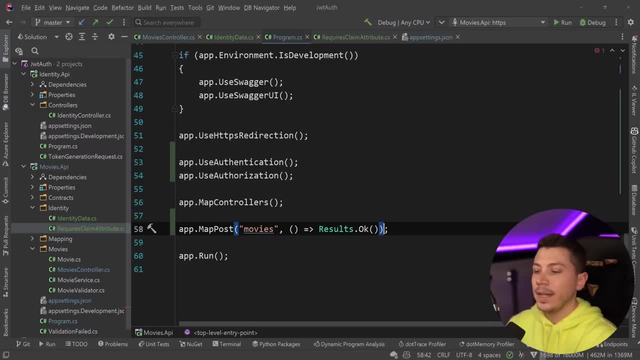 post and let's have a movies endpoint post. and let's have a movies endpoint over here and return results: dot okay over here. and return results: dot okay over here. and return results: dot okay. for example, now you can pass down an. for example, now you can pass down an. 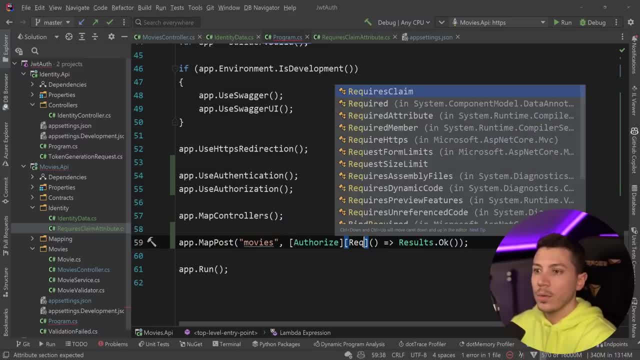 for example, now you can pass down an authorized attribute over here and all authorized attribute over here and all authorized attribute over here and all of that will still work, or requires of that will still work. or requires of that will still work, or requires claim like that is just valid. c sharp. 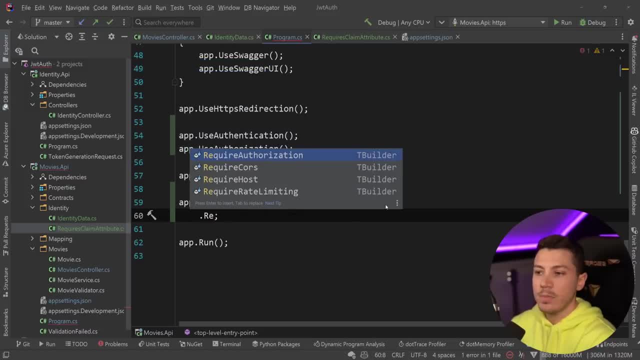 claim like that is just valid c sharp. claim like that is just valid c sharp. however, in minimal aeps we actually, however, in minimal aeps, we actually, however, in minimal aeps, we actually prefer the extension method approach. so prefer the extension method approach, so prefer the extension method approach. so we're gonna say: require authorization and 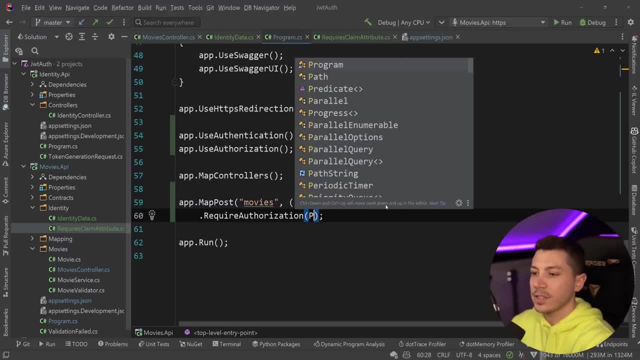 we're gonna say: require authorization, and we're gonna say: require authorization, and you can create your own extension. for you can create your own extension. for you can create your own extension for the claims and everything. but you can the claims and everything. but you can the claims and everything, but you can pass down like a policy over here. you 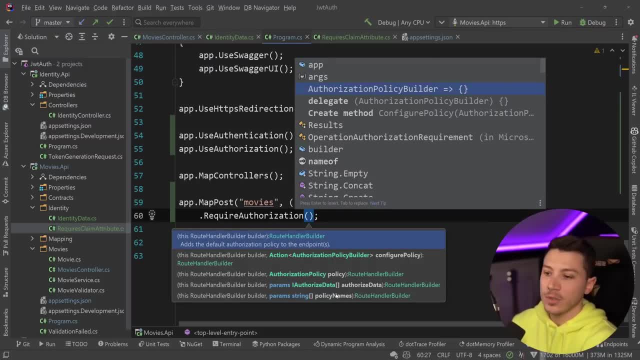 pass down like a policy over here. you pass down like a policy over here. you can see all the parameters you can pass. can see all the parameters you can pass. can see all the parameters. you can pass down multiple policy names as well, but down multiple policy names as well, but 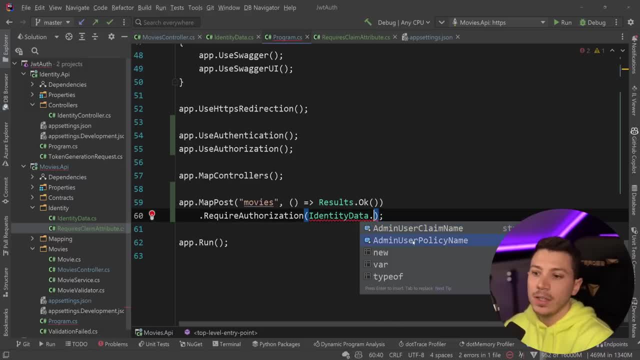 down multiple policy names as well, but in this case, if i just say identity data, in this case, if i just say identity data, in this case, if i just say identity data- dot admin user policy name, this will be dot admin user policy name. this will be dot admin user policy name. this will be the same thing as having the attribute. 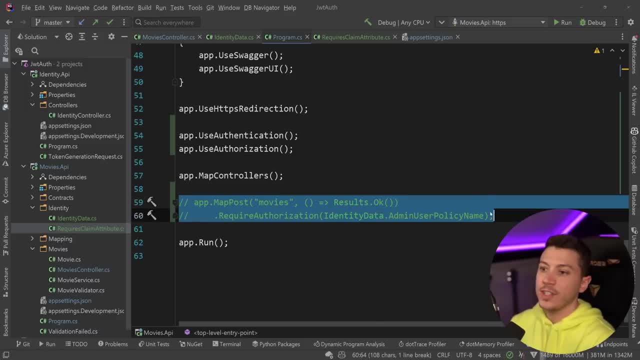 the same thing as having the attribute, the same thing as having the attribute with the policy name. now the last thing with the policy name, now the last thing with the policy name. now the last thing you might be interested is actually you might be interested, is actually you might be interested is actually swagger support, because if i just go, 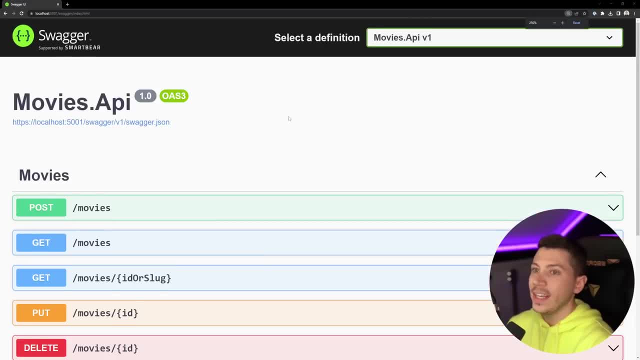 swagger support because if i just go swagger support, because if i just go ahead and i run this api as it stands, i ahead and i run this api as it stands, i ahead and i run this api as it stands, i can go in swagger and even though i can, 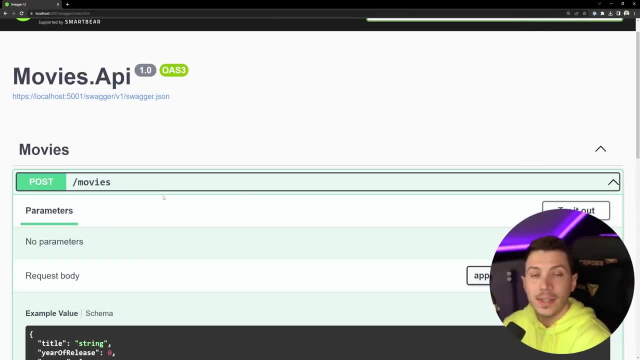 can go in swagger. and even though i can can go in swagger and even though i can see all of my endpoints, i can't see a see all of my endpoints. i can't see a see all of my endpoints. i can't see a way to actually authenticate with the. 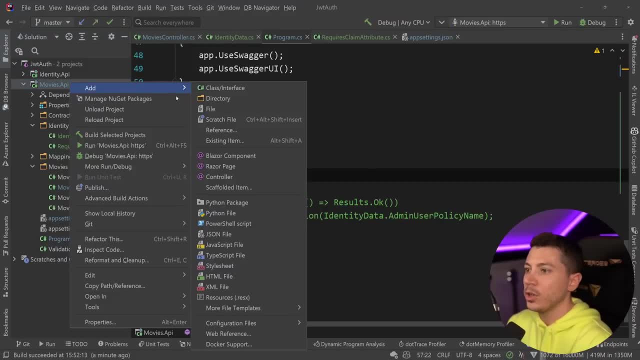 way to actually authenticate, with the way to actually authenticate with the token. so how do i do that? well, it's token. so how do i do that? well, it's token. so how do i do that? well, it's actually quite simple. all i'm going to actually quite simple, all i'm going to. 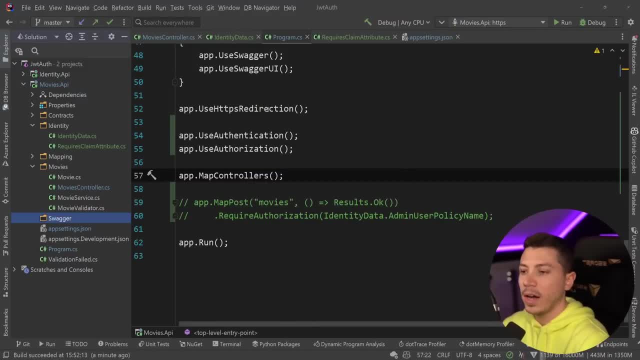 actually quite simple. all i'm going to do is create a new directory called do is create a new directory called do is create a new directory called swagger, and i'm going to bring two files swagger and i'm going to bring two files swagger and i'm going to bring two files in here. the first one is called: 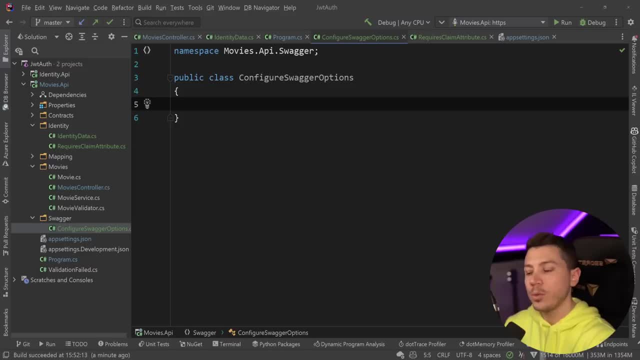 in here. the first one is called in here. the first one is called configure swagger options and we're configure swagger options and we're configure swagger options and we're gonna contain all the swagger related, gonna contain all the swagger related, gonna contain all the swagger related options in here, and this will need to. 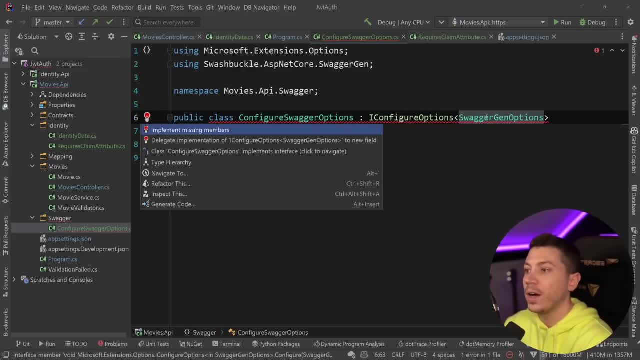 options in here and this will need to options in here and this will need to implement the i configure options and implement the i configure options and implement the i configure options and then have the swagger gen options file, then have the swagger gen options file, then have the swagger gen options file in here, implement and we have the. 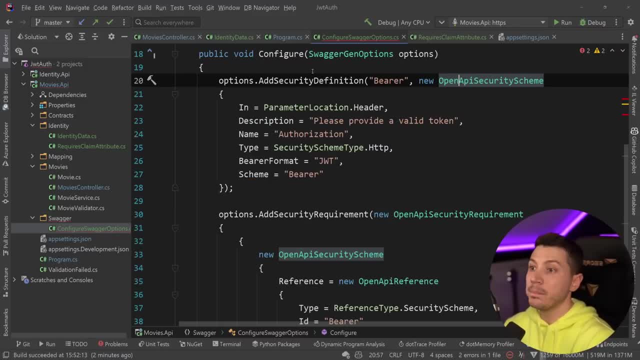 in here implement and we have the in here implement and we have the configure method in here and i'm not configure method in here and i'm not configure method in here and i'm not gonna bore you with typing all of this. gonna bore you with typing all of this. 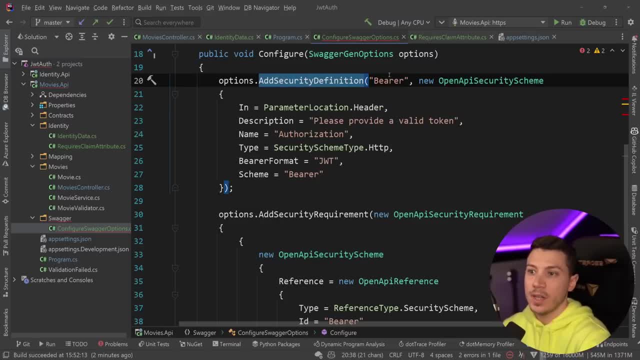 gonna bore you with typing all of this, but ultimately what you need is a, but ultimately what you need is a, but ultimately what you need is a security definition, and we say that this security definition, and we say that this security definition, and we say that this is a bearer token specified, that is. 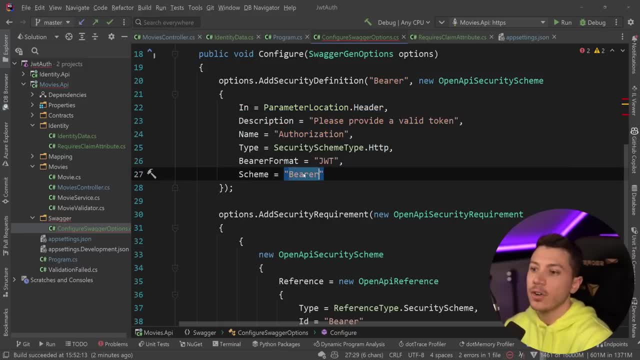 is a bearer token specified. that is is a bearer token specified. that is located in the header authorization. located in the header authorization. located in the header authorization: http jot bearer. everything is here, same http jot bearer. everything is here, same http jot bearer. everything is here, same with the ad security requirement and. 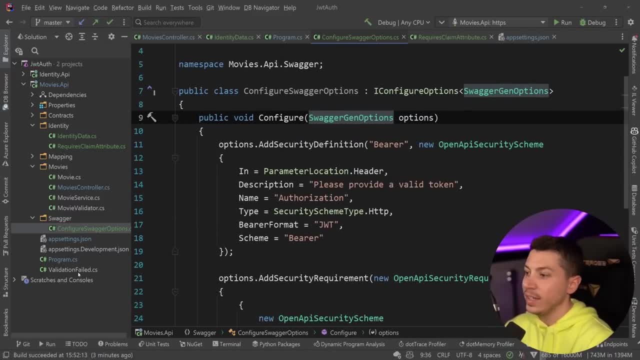 with the ad security requirement and with the ad security requirement and really that is it from that front and really that is it from that front, and really that is it from that front. and then once you have that, you actually, then, once you have that, you actually, then, once you have that, you actually need to register it in the programcs. 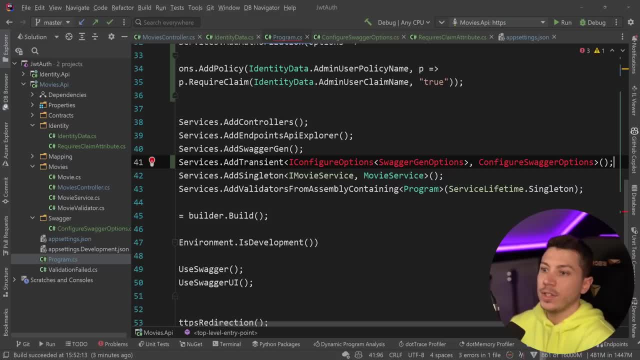 need to register it in the programcs. need to register it in the programcs. so all the way up here we're gonna go. so all the way up here, we're gonna go. so all the way up here, we're gonna go here and register the i configure options. 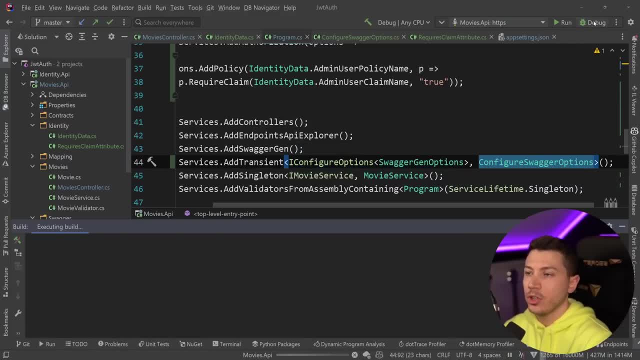 here and register the i configure options here and register the i configure options interface with its implementation and interface with its implementation and interface with its implementation. and once that's in place, all i'm going to, once that's in place, all i'm going to. once that's in place, all i'm going to do is just run it. and now, if we go back, 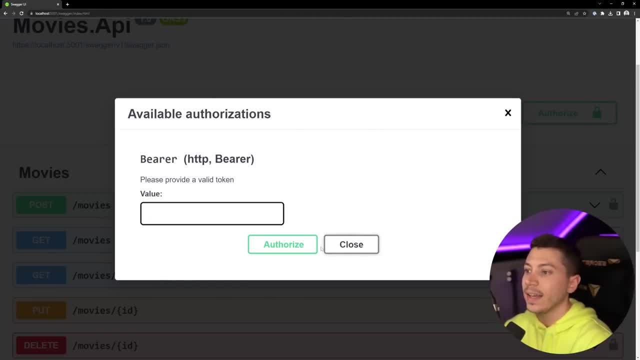 do is just run it. and now, if we go back, do is just run it. and now, if we go back to swagger- as you can see, i have this to swagger. as you can see, i have this to swagger. as you can see, i have this authorized button which i can click and 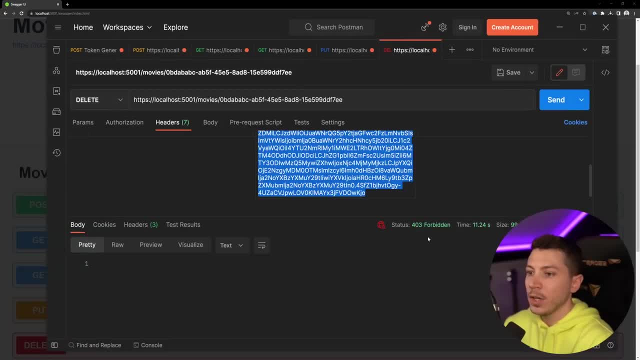 authorized button which i can click. and authorized button which i can click and provide the json web token. so we're provide the json web token. so we're provide the json web token. so we're gonna go all the way back here. copy. gonna go all the way back here. copy.